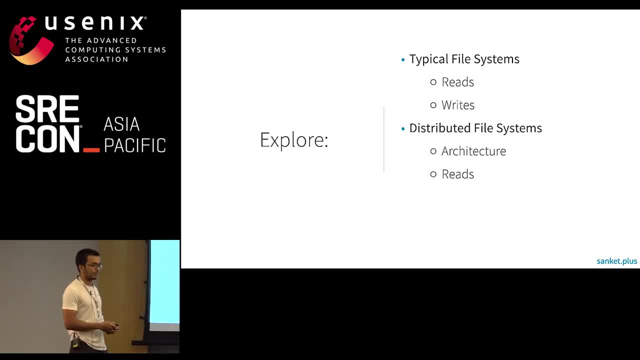 see if you want to read a file in the distributed environment, how would it look like? Again, the writes And, as I said, the best way to learn anything is by doing it. So you can, I'll introduce you to a tiny, cute little distorted file system that will see how does the read and 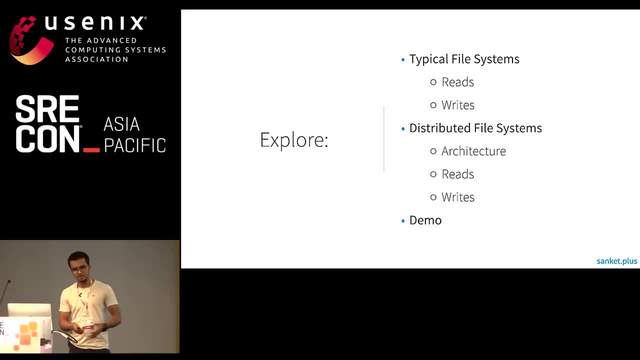 writes will look like in that one, so things will make more sense if you actually see it happening. here's what we are not going to explore. we won't be exploring any particular file system- let's say ext4, ext3, hdfs or any particular file system- but the architectures that we'll be seeing will be. 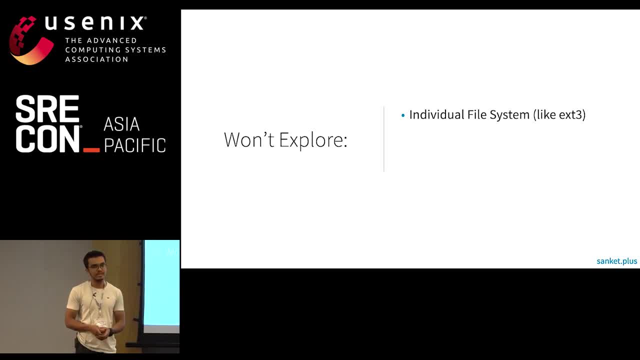 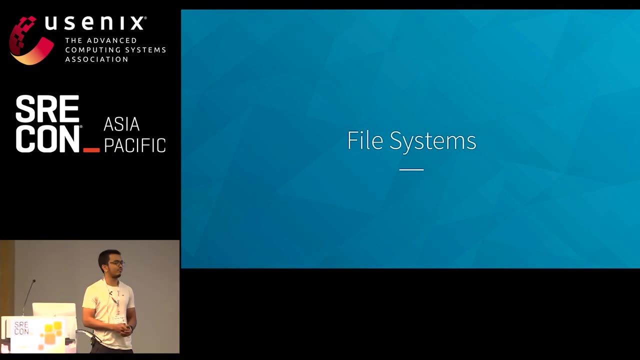 generic enough to be comparable with most file systems that exist today, so i hope that wouldn't be a problem. uh, conceptually, most should be relatable. and, of course, answer to the ultimate question. uh, we all know the answer to write, so let's get started. uh, what are? what are file systems? 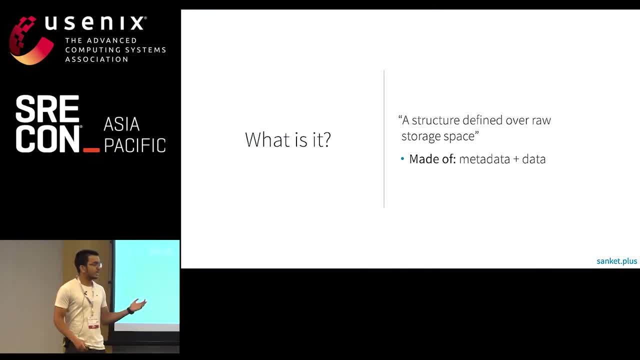 to tell it in a single sentence or simple, oversimplified way: a structure defined over a raw storage space. what is raw storage space? your storage devices, uh, hard drive, pen drive, you, or memory cards? So we'll define some structure over it so that we can utilize it better. 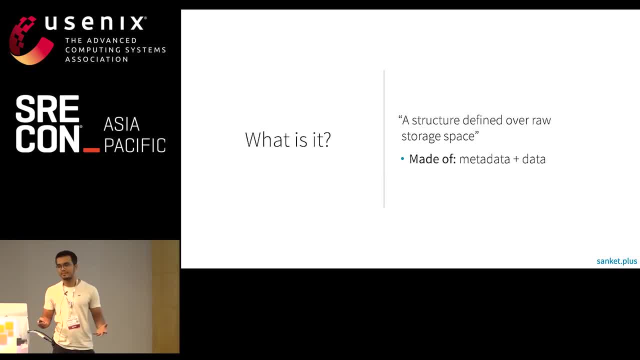 If you want to classify it on a really high level. it is made of data and metadata. We'll see how does it look like, But before we see what does it look like, let's try to build our own file system. You have a device and you have an API. 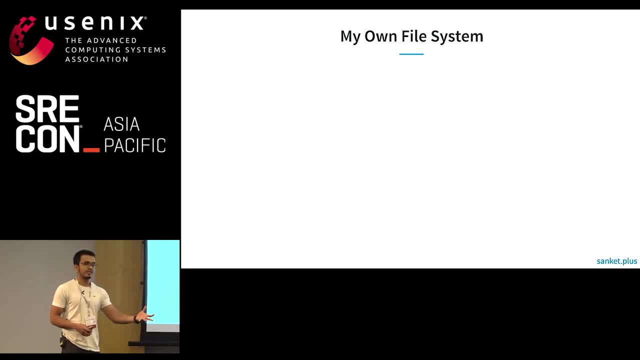 What that API can do for you is you can give it an address on the disk and you can read back the content from the address. So this is what you have: a storage device and you can read content from any random place. Now let's try to build our own file system. 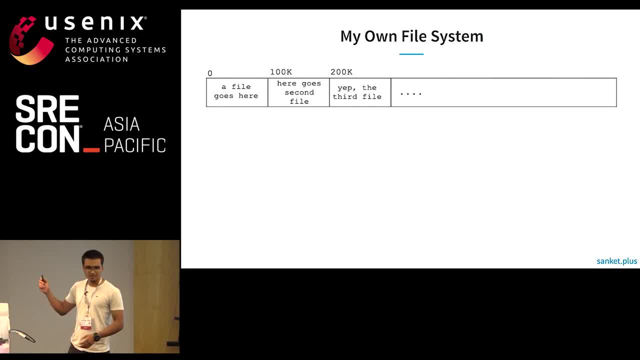 before we explore what existing ones look like. Really basic version. we divide storage space into fixed blocks, In this case 100K. So how do you use this up? You want to put file. you put it at every 1,000K offset. 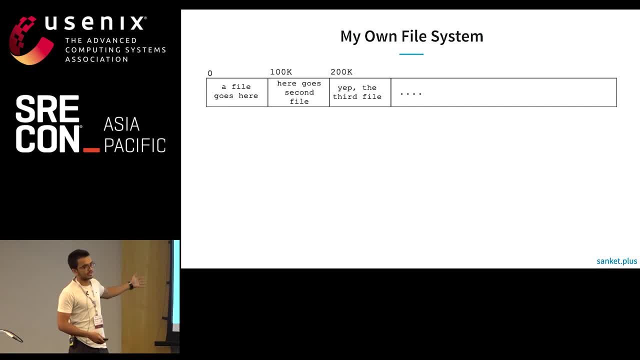 Sorry, 100K. So you want to access the first file, you access it at zero offset. You want to access third file, you go to 200K and access that file. Really basic, but it works. There are some limitations. First being: you cannot put a file that is more than 100K. Yes. Second being: you might end up wasting some space if the file is smaller. But good for, I guess, If you want to make it a bit better resource utilization instead of going fixed blocks. 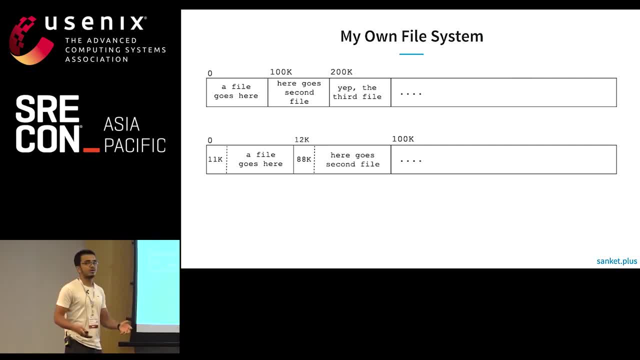 what we can do is: let's not go fixed blocks. We first, at the start of every block, we put the file size first, Say 11K, and then you put the file. When it ends, you put the next file size. 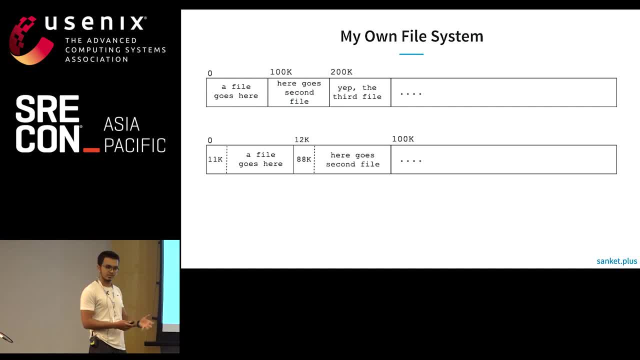 Then you put the content, It gets a bit better than the first approach. Say, you are now having variable size files, You can have files of varying lengths And you're also not wasting space. So it works better than the previous one. If you want to make it a bit better, more along with this: 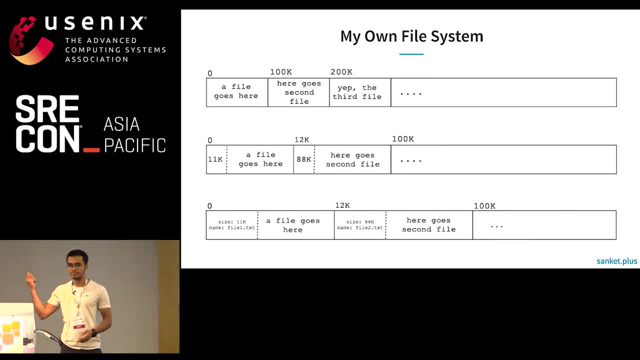 you can also put the content Along with the size. what you can do is put maybe file name, So along with the size. you can call it file1.txt, foo, file, whatever name can be put in, And if you want more metadata around it, 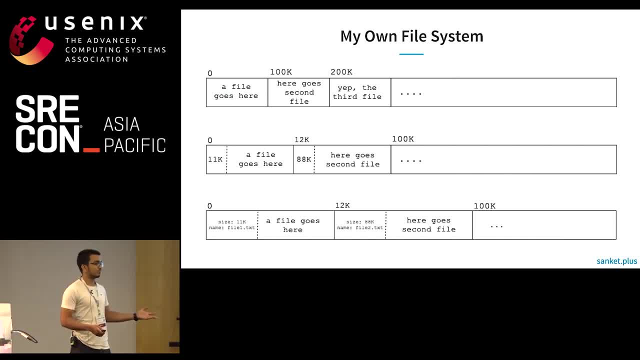 you can also put who owns this file, when was it last accessed, when was it created, things like that. So if you see where we are going with this metadata approach, it might sound familiar to you, And I know. So. this is the kind of metadata that I know will contain. 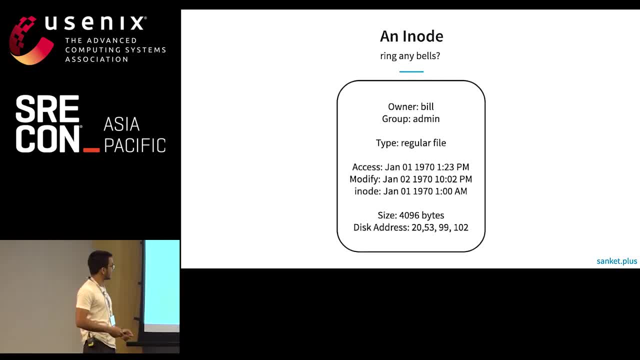 If you don't know what an inode is, here's what it looks like. So what inode is? it is basically a structure or some sort of metadata that the file will have. So some of the things that generally will go in is: who owns this file or whatever it points to. 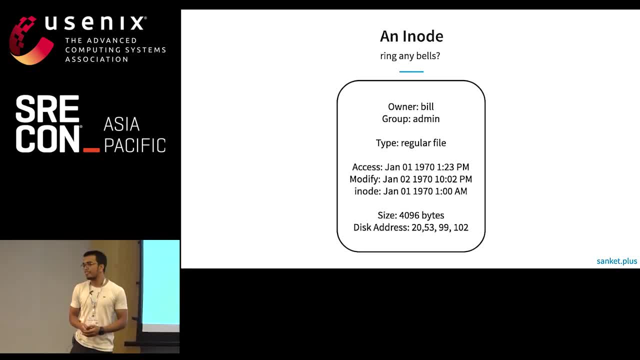 who is the group that the user belongs to or the file belongs to, the important one being our type. that what kind of data the inode is pointing to, Say, file, directory, link device, some timestamps and, of course, in the end sizes, that how big. 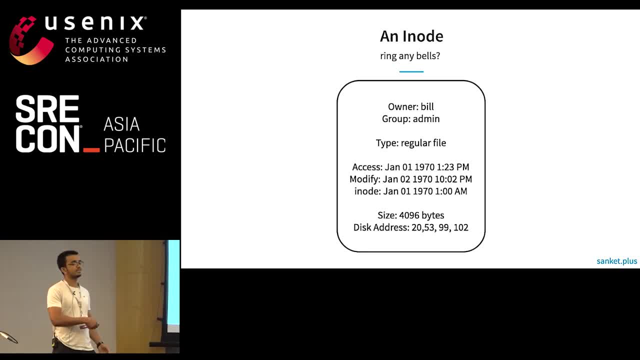 And the most important will be disk addresses. That is, where does the actual data is located at. So do you think these are the metadata, say, for a file? Do you think anything obvious is missing? Maybe file name, like we have all the things but not the file name. 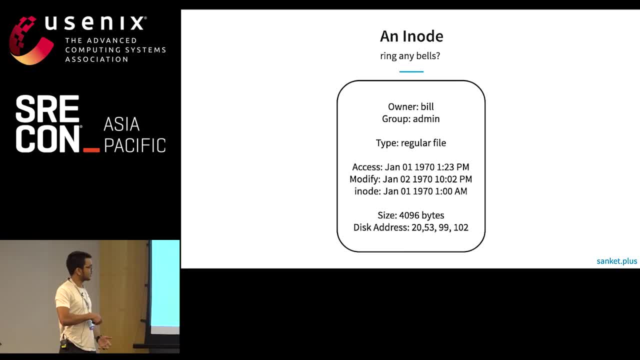 Do you think it is missing? It is not, So we don't put file name in here. We'll see where does it go. Let's take a look. If you've got an inode for a file, what will it look like? 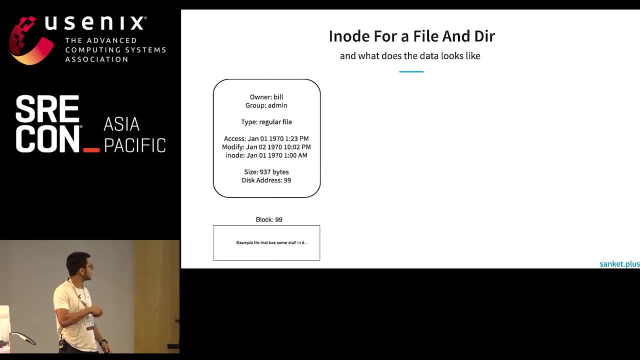 So all things will go in as usual owner groups. some timestamps. The type here will be differentiating. That will be a regular file, The size will be there, disk address And if you want to read the content of the file, 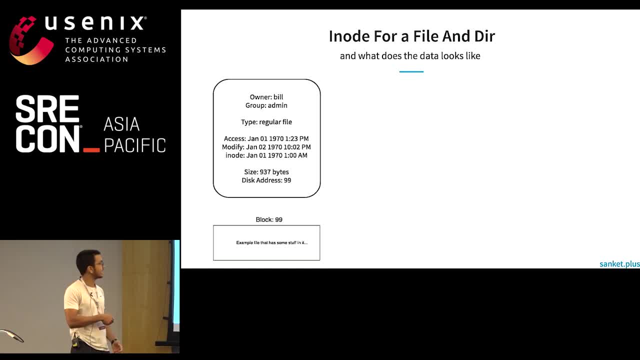 you'll go to disk and you'll access the block number 99. And whatever the block has containing contains that is, your file's content. So this is what it looks like for a file. really simple, Nothing fancy going here. 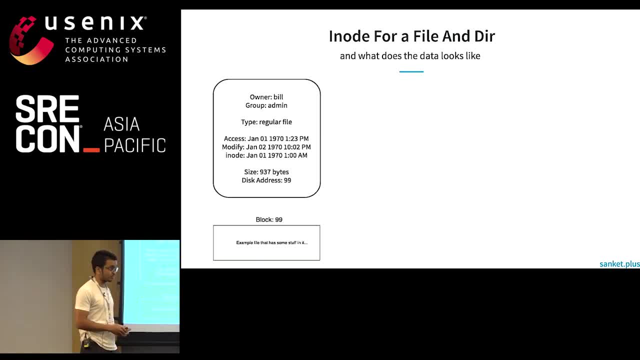 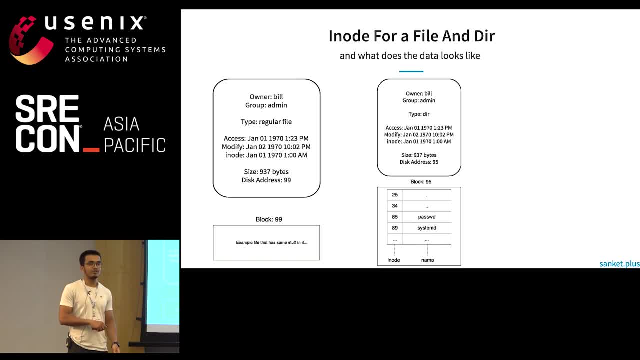 Let's take a look. If it is for a directory, of course it's going to be a file. Let's take a look. If it is for a directory, of course it's going to be a file. Let's simplify it a bit and put it in a tabular format. 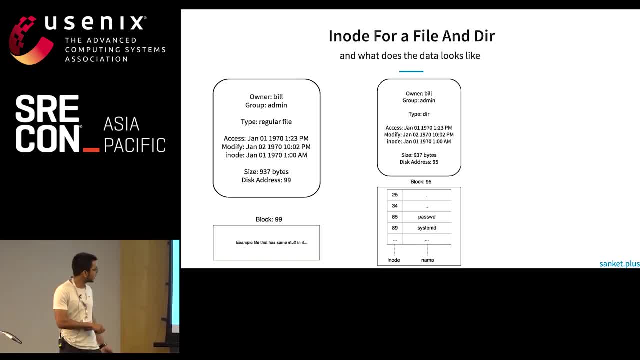 We'll have two columns, the first being the inode numbers. what are the contents of the directory and inodes for that and what do you call it? So here is the place where your name will be going. So say, if a directory has inode 85 and you want to call that file, 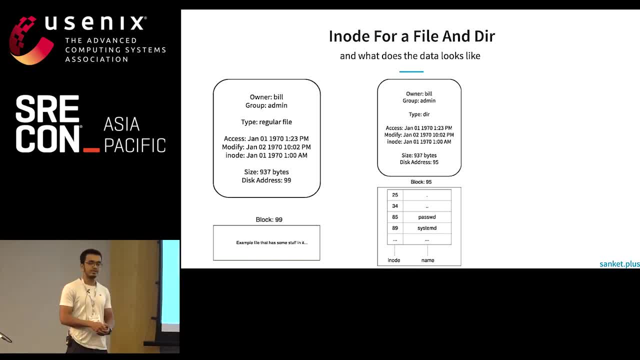 or directory, whatever it is- password. so here is the place where you will be putting the name. Now, this is what it will be looking like. Now, this is what it will be looking like. Now, this is what it will be looking like for a file and a directory. 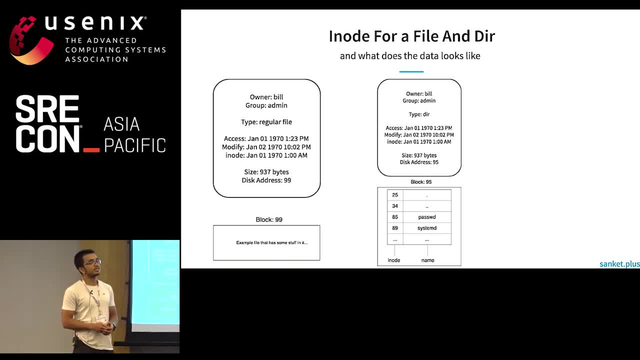 Now, having understood this, let's also try to understand something that we use every day, that is, links. We may have heard of it: soft links, hard links. Let's see how does it actually look like and how does it work. So we have a file here called password, and inode number is 85.. 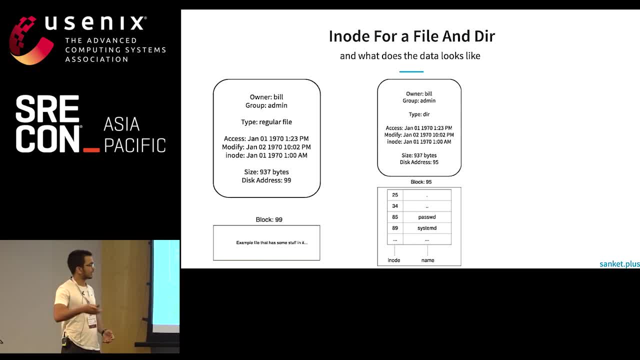 Now, in the same directory, you want to create a link, You want to create a new file called users and it should be pointing same content in as password. really simple, Because it's a table, we add one more entry, inode being 85,. 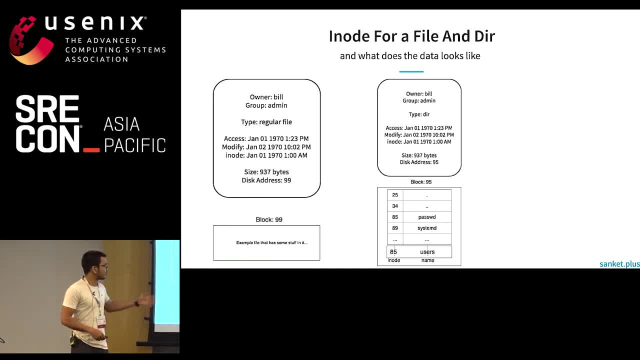 and in the name column you put users. So in the directory listing you got two files. One is called password, one is called users and because they have same inode number they point to same content. because you know where does the data is stored at. 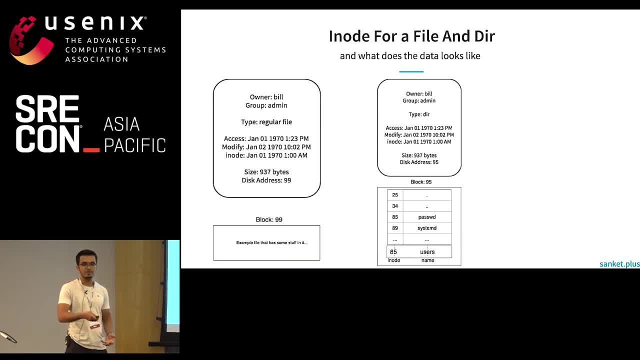 It's stored in inode. So both the files point to same disk blocks. and there you go. You have a link, You have a hard link. Now how will a soft link look like? Well, in case of soft link, you won't be putting it in a directory entry. Instead, instead of the disk address, you'll be putting whatever the link it is pointing to. So that is why, in case of soft link, you can put anything instead of disk address. Your file can be pointing to any random. it's just a string. 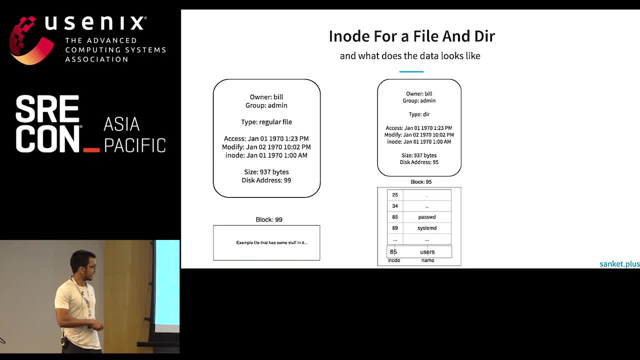 You can put anything and it may not have to be existing. Well, in case of hard link, this inode number will be existing and file system will ensure that hard link can never be broken. So that is soft link and hard link. 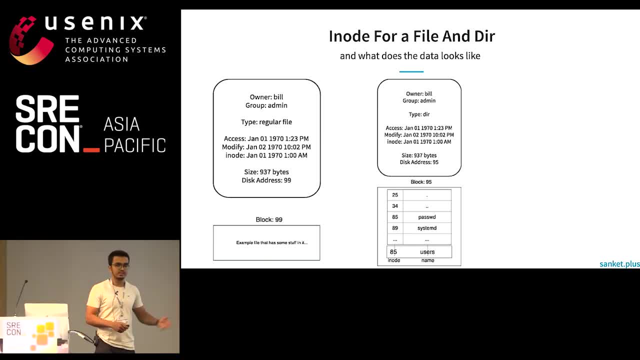 Now systemd is a directory. Let's take one more example. It's a directory and you want to create a hard link for directory. So, if you're following the structure and the way that things look like, what you can do is you create one more entry in the directory listing. 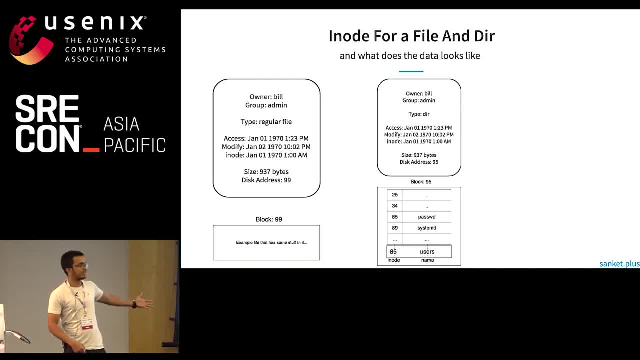 It's just a table Entry. inode number will be 89, and you want to call it systemd-link. Logically, you can put it right. There's nothing stopping you. It makes sense. You're just making one more entry. 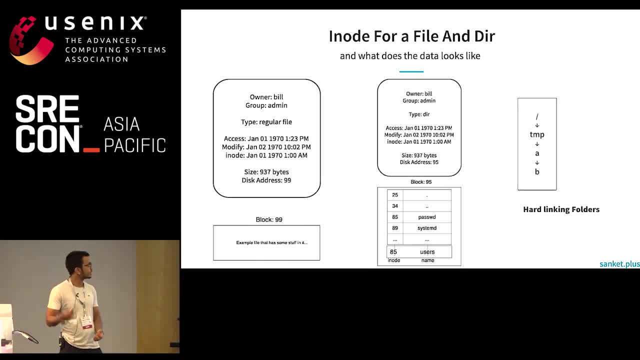 But why not? Systems won't allow you to. Why not? Let's take a look. Why is hard linking not allowed for folders? Say, you've got this example structure: You have temp directory. Inside temp you've got A. A is a directory and inside A you create a directory called B. 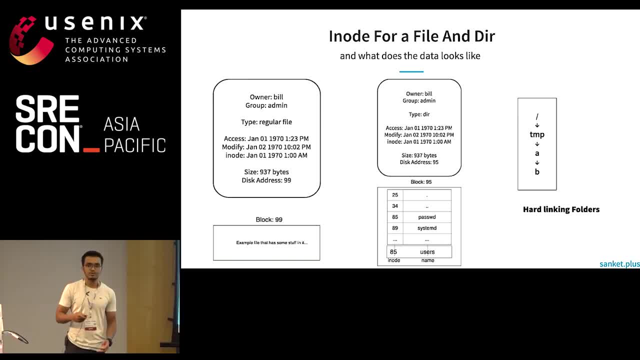 So temp A, B, all are directories. Now let's try to create a hard link called L In folder B. L will be pointing to A. This is just an example, So it can be created if it was allowed. 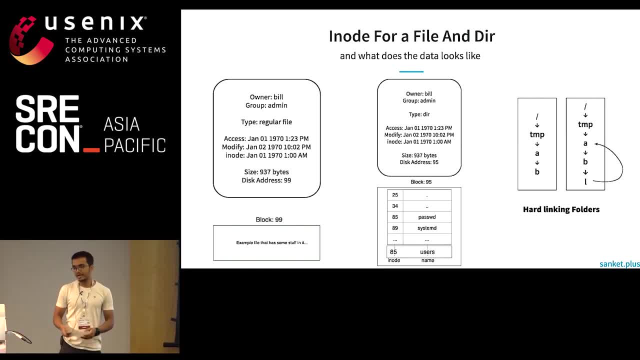 Now what's the problem here? Say you wrote a script that recursively lists out all the contents of the directory. So your script starts: It lists out content of temp, What it sees: It sees A. It lists out content of A. 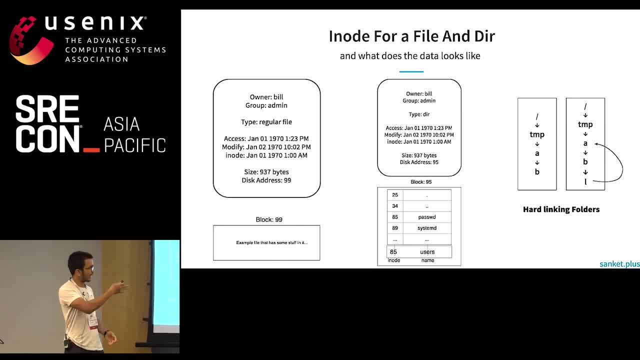 It sees B. It lists out content of B. It sees L. Now L is linked to folder A. If it lists content for L, it will be seeing B again. In B, it will see L. In L it will see B. 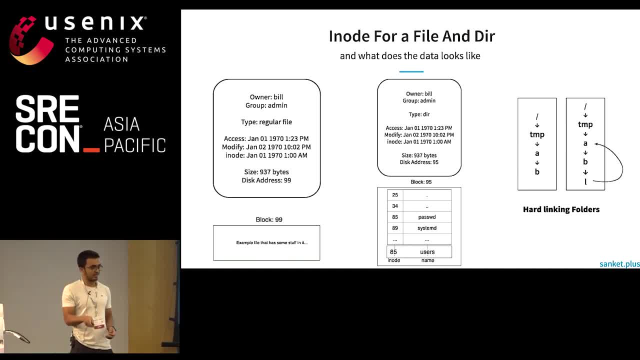 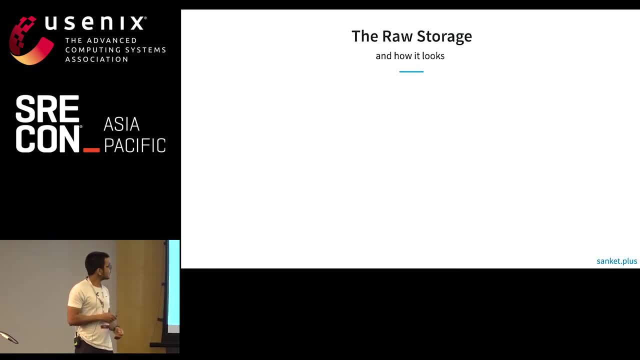 So you see there's a loop here, So your script can go an infinite loop And logically this thing doesn't make sense. So that is why hard links are not allowed. Now, this was inode. This was data blocks. We are talking about file systems. 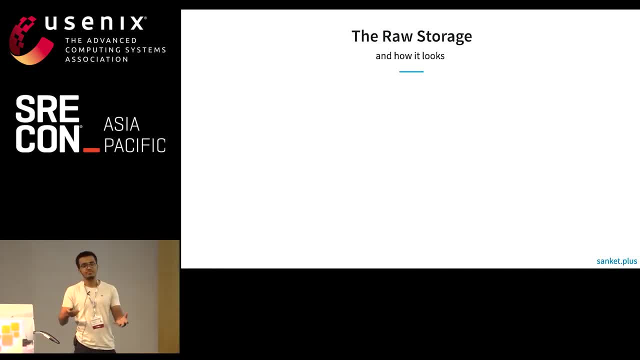 So where does it fit into your raw storage space? Where does it fit in? So this is the overall simplified structure, The rectangle being the whole of your storage device. We'll be partitioning it because that's what we said. What is a file system? 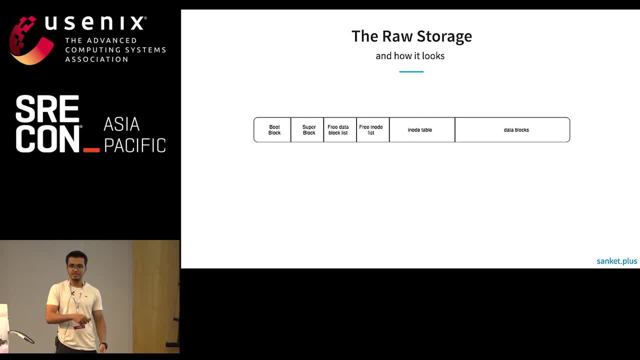 That is a structure defined over our storage space. So this is the kind of structure that we define, or the normal file system would define Data blocks that will actually be containing data. We'll have an inode table where the inodes that we just saw will be going in. 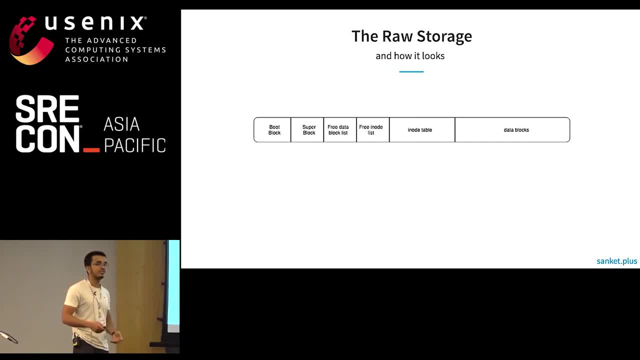 We'll also be maintaining two more lists called free block list and free inode list, Because if you want to create a new file or if you want to extend a file, you need free inodes or free data blocks. So here's a handy list that you will be maintaining so that you can quickly grab some free data blocks or the inode. 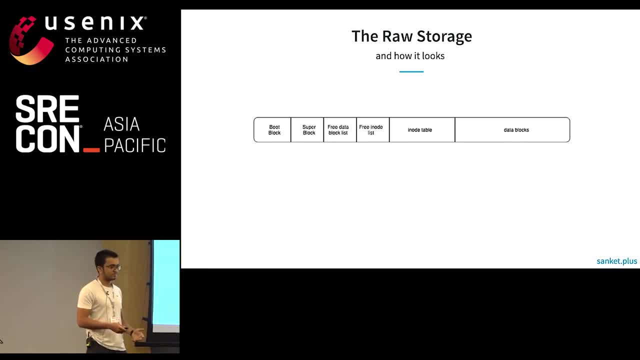 There will be a super block. Super block is metadata of your whole file system, That is, how many inodes are there, how many blocks are there, what is the utilization, things like that, What is the block size? And there will be a boot block. 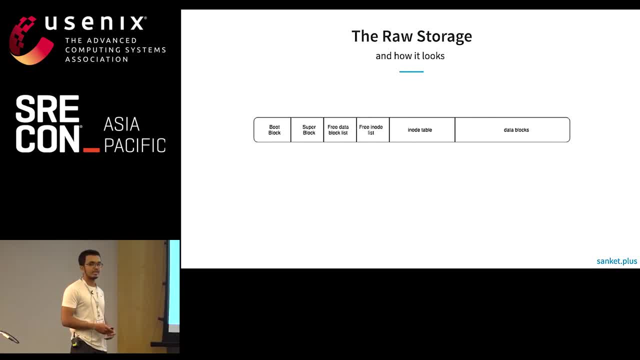 So if, in case, your disk or the file system is bootable, then the booting instruction would go there. So this is the overall picture where your things would go in. Now let's take an example. You got a file system that has data block size worth of a million bytes. You have divided into thousand bytes block, So you have one thousand blocks. Now how many files you can create? You want to create a million files that is one byte long. One million files that has one character. Can you create one million files? 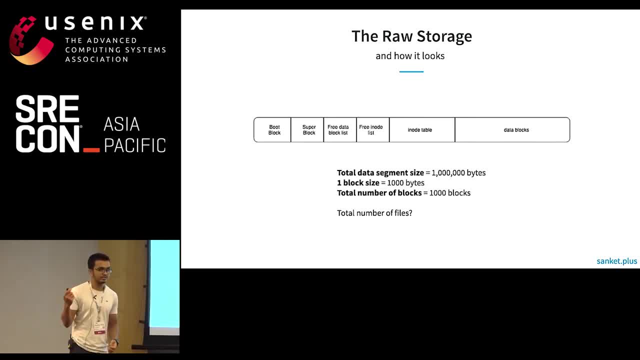 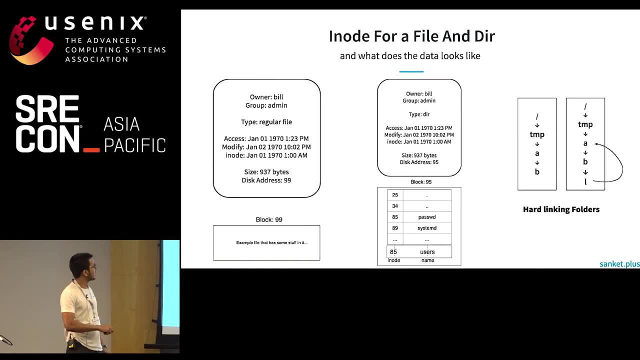 You got space for that. You got one million bytes. Can you create one million files? No, you cannot. Why? Because if you go back and look at the inode, you see in inode you specify a block's address. So each file, at least, will be using one block. 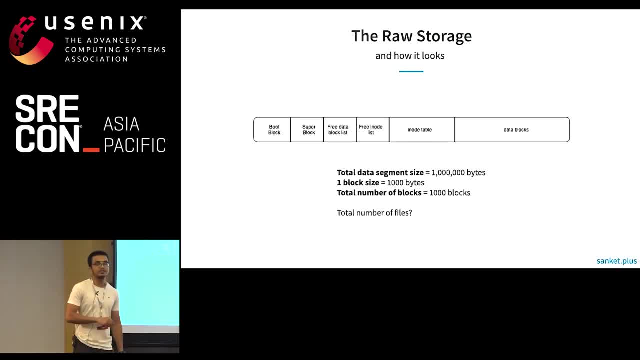 So in this case, each file will at least be using thousand bytes. Whether it contains one byte, five bytes, ten bytes, doesn't matter. Thousand blocks will be allocated to one file. So how many files you can create? Thousand, Thousand. 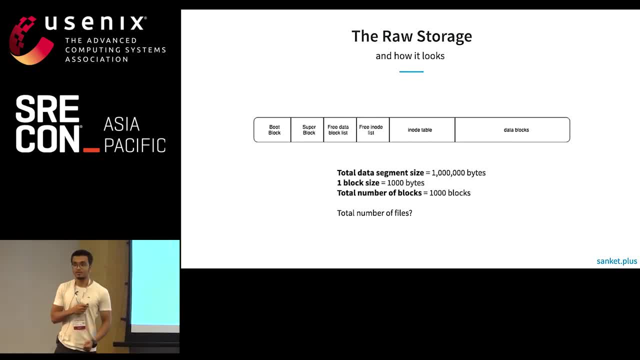 But can you? Can you create thousand files? Well, the answer is: depends, Depends on what Inode table. So you see, even if you have thousand blocks, you may not have. This is a fixed size structure, as we said in the beginning. 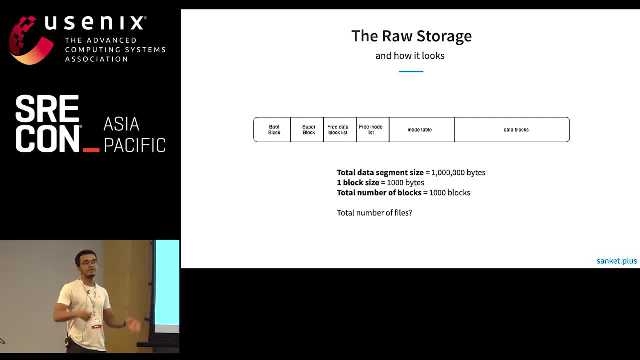 This is a structure defined across storage space, So the inode table is a fixed structure, So it may not have space for thousand inodes. So it really depends. If you have less than thousand inodes, you cannot create thousand files. Now, these are. 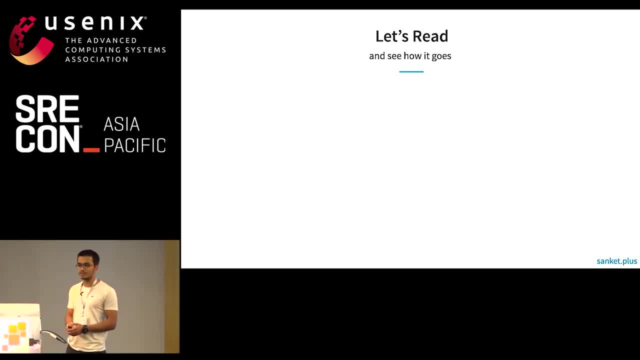 This was the overall picture. Now we promise that we'll be seeing how will the read look like and writes will look like. So let's take an example. Let's try to read a file that we all know Slash, etc. slash password. 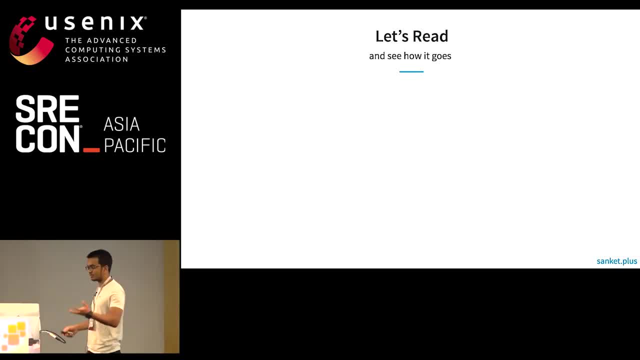 We all know this file. What you want in the end is: whatever the content it contains. What we know about is the overall structure And inodes and data blocks. we all know what goes in Now: slash, etc. slash password. What is slash? 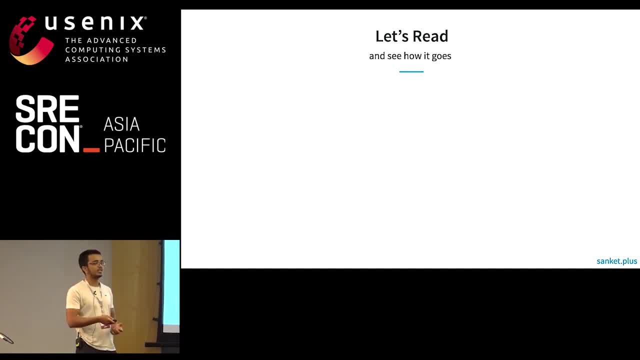 It's a directory, It will have some contents in it. So if it is a directory, there has to be an inode to that, Because all files in directory have inode numbers. So inode for directory slash is two, Because you need some place to start. 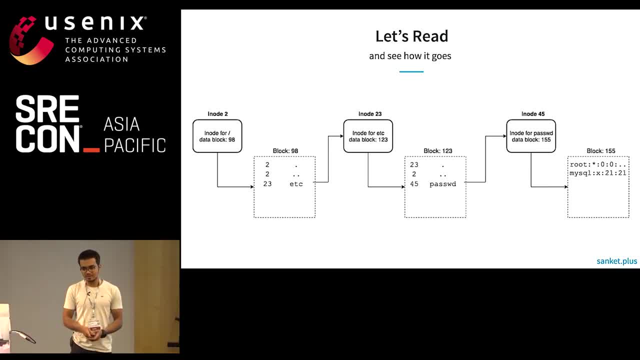 You want to list out content for directory slash, You need some place to start, So inode two is the place you start. Now why inode two? Because inode zero basically means null Null value for inode. Inode number one is reserved for listing for the corrupt blocks. 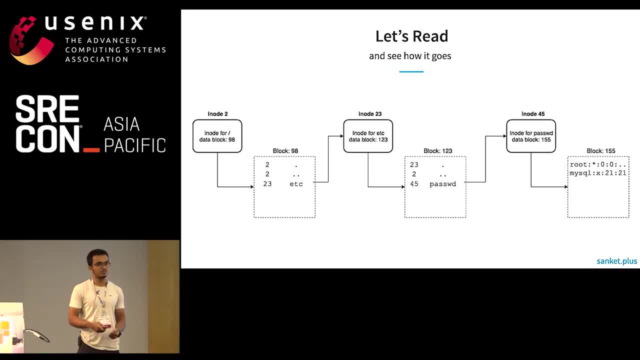 Like you, maintain the list of corrupted disk blocks. So next logical choice that was available was inode two. This is more sort of a convention, It's not a fixed thing. So this is the convention that the movie file system will use. So there you go. 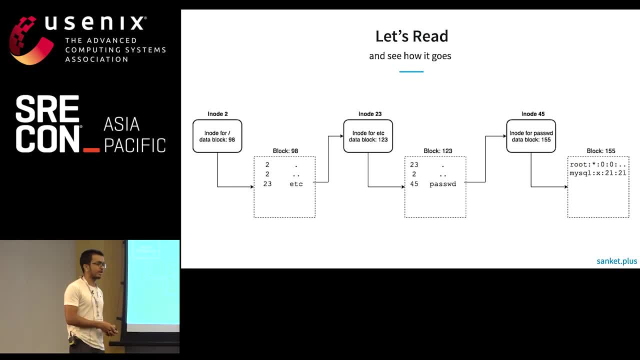 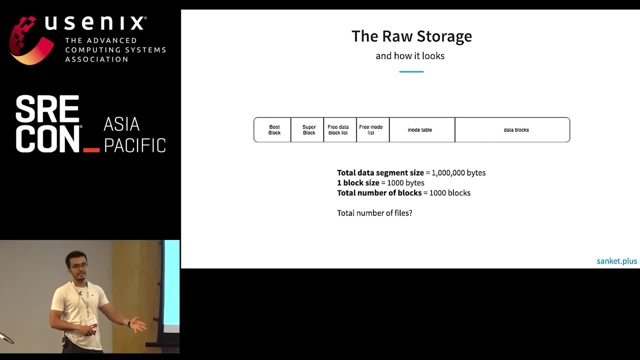 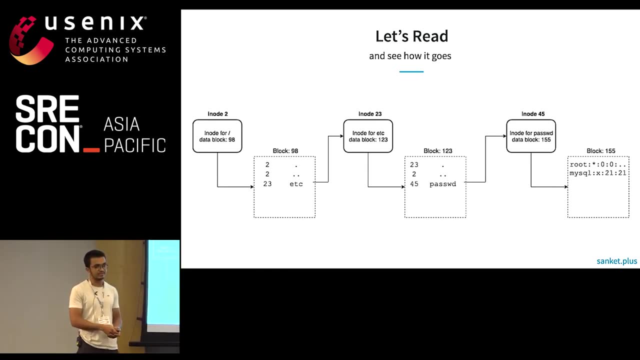 You have a place to start. You know slash for inode, for directory, slash is two. So what will you do? You'll go back to the inode table. You'll fetch the inode two. Inode two will find that data block associated is, in this case, for example, 98.. 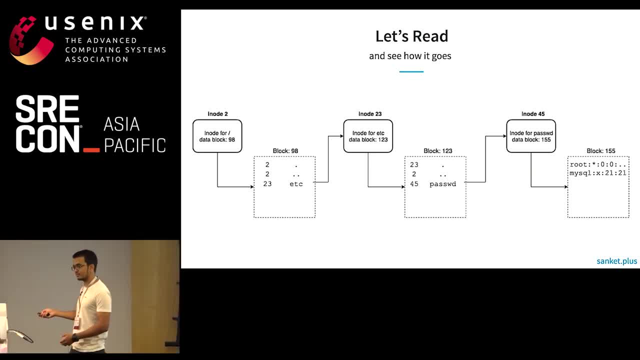 So you'll go to the data block section of your file system, You'll fetch the block number 98.. And you'll list out the things. Now, what are you looking for? Slash, etc. slash password. So you'll enter that. So in the directory listing in the table, you'll be looking out an entry for etc. 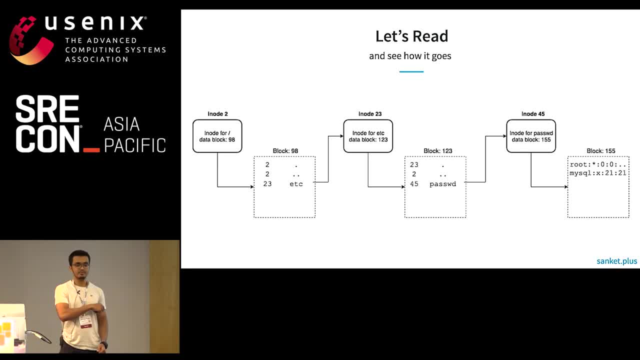 Now for etc. the inode number happens to be 23.. So again, you'll go back to the inode table. You'll fetch the inode 23.. The inode 23, it is for directory etc. So if you list out the contents, it should be contents for directory etc. 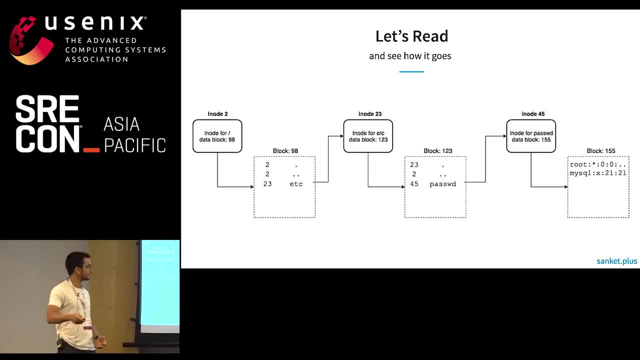 What are you looking for? You're looking for password, the next component in the path. So the password- you'll be seeing that inode- is 45. You go back to the inode table. You fetch the inode 45. You see what data block is associated. 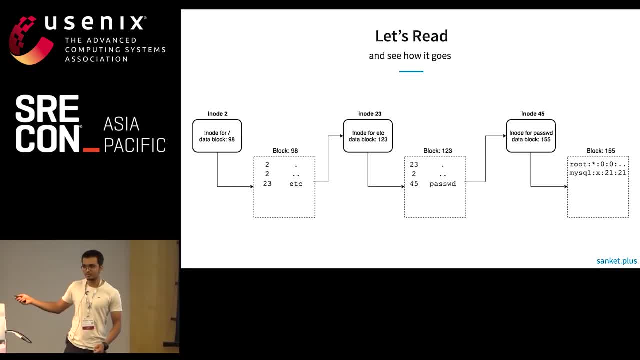 In this case it was 155.. And finally, when you go to the data block section, you fetch the data block 155.. And there you go, You have your files content. So this is how a read would look like. Now let's talk about writes. 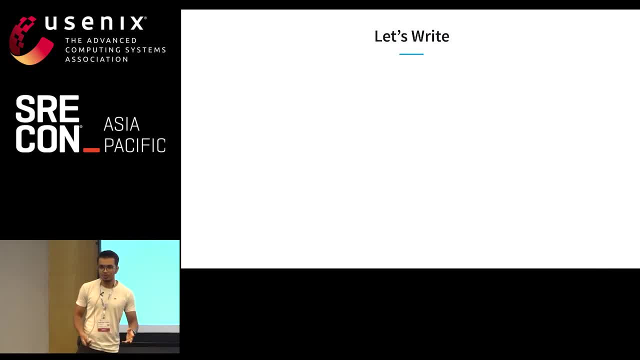 So you want to write to a file, So obviously to write, you will be writing it to some data block And, as we just saw, to get the data block you need the inode number for the file. So you'll be doing the same thing. 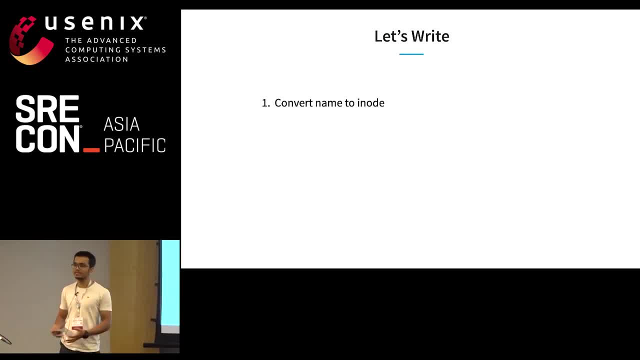 You'll be converting the file name to the inode, like we did with the reads case. So you convert, You get the inode number, If in case, the file was a new file, that nonexisting file, so you know where to go to. 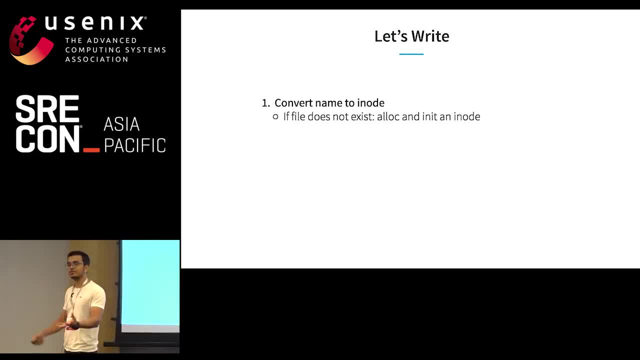 You have to create a new file, so you'll need a new inode. You need new data blocks. You know where to find them right. So if the file is nonexisting, you'll locate a new inode from a free list. If file is existing, you need to get the data block. 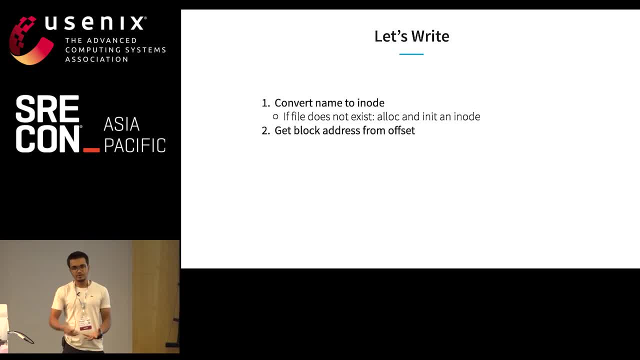 So from given offset, say you want to append to a file, you'll get the last data block. If you want to append to a file, you'll get the last data block. If you want to add something in the beginning of the file, you'll get the first block. 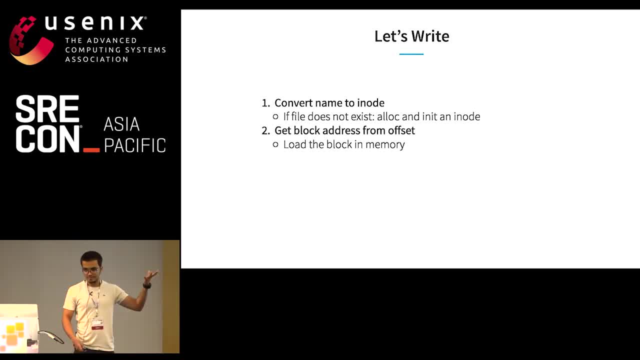 You load that block into memory Because the block in the disk. you load it into your memory. If you want to append to some file, if the block doesn't exist- like you're extending the file- you have to allocate a new block. 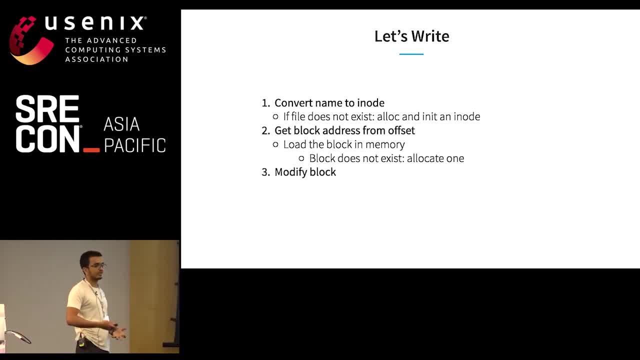 So in that case you'll allocate a new block And finally, when you have the block in the memory, you do whatever you want: You change, append whatever you want to do And finally put it back to the disk. 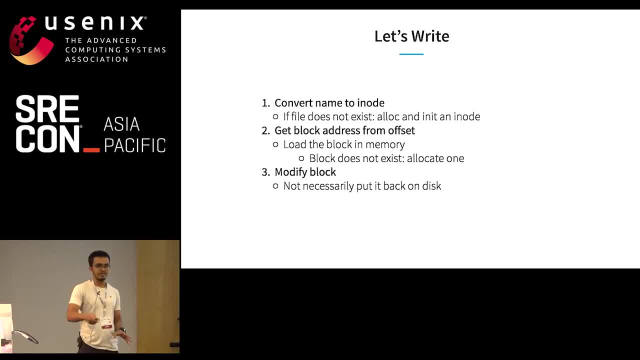 So you do write call And you assume that your block has been written to the disk. But is it really, Not really? When you write anything to a file, it is not immediately written to the disk, the actual storage device. What your OS does is, even if you write it, it will kind of hold it for a while in memory. 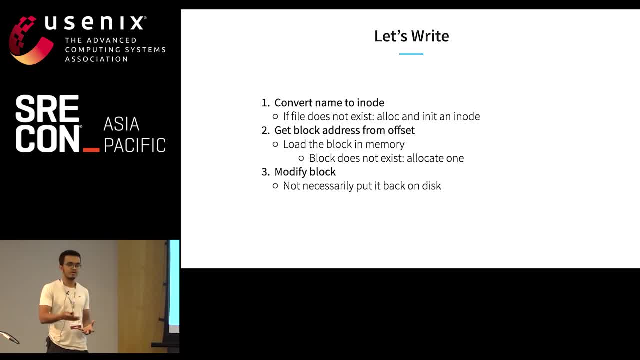 So that when a bunch of enough writes has been done on the disk, it will match all these things together and later put it to the disk in a flush so that it can optimize things a bit. So this is the reason why in older days you've been seeing these warnings that you should 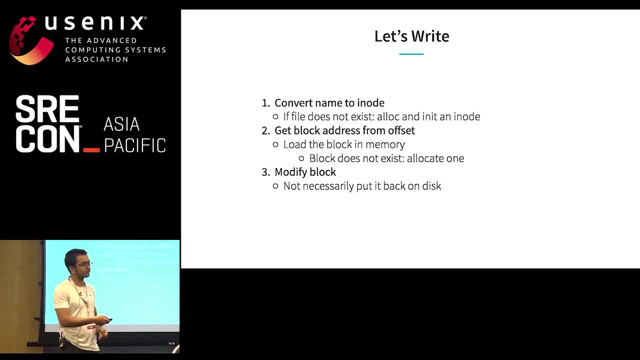 not just pull out a USB device, or you should safely remove the device. This is the reason why: Because you may have written things, your OS might not have flushed those blocks into your actual storage device. So this is why your OS advises you to do safety remove so that it can do all the pending writes. 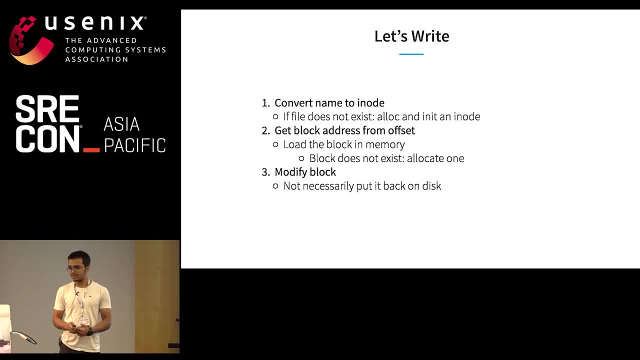 to your disk, And this was the reason why you've been seeing those warnings. Now, if you look at the rest of the data, you'll see that there are a lot of things that can go wrong. Now, if you look at the write process, you see it's a multi-step process, right? 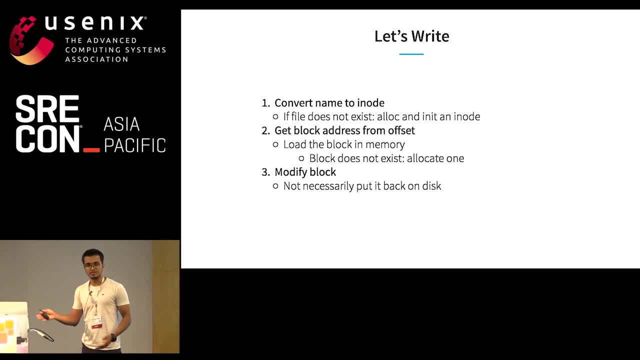 Things can go wrong when you are doing this: Power cut, OS crash, things like that it may happen, And if you were to get stuck somewhere in between- that you were on step two or somewhere in between and this thing happened- then your file system may go in an inconsistent state. 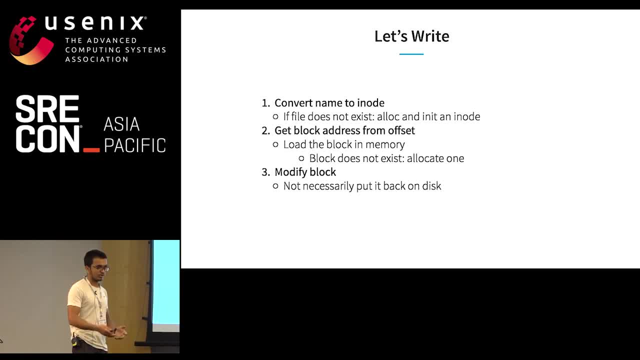 You're going to do something, but you didn't finish it, so your file system is not consistent anymore. So to overcome these problems, new version of file system is needed. So this is the first step. The second step is to introduce the concept of journaling. 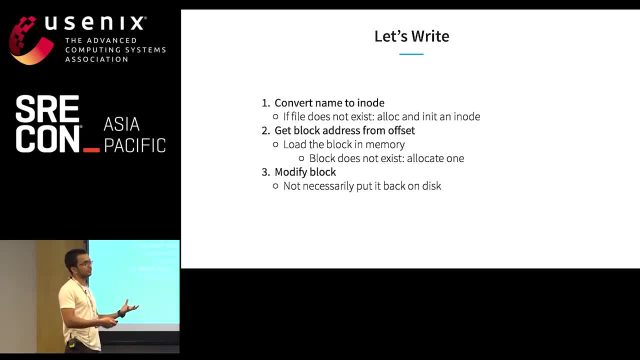 What is journaling? Basically the structure. we saw there's one more section for journaling. So in journaling what you do is you write what you're going to do. You are going to do these three steps. You first write that I'm going to do these three steps and then you go and actually do it. 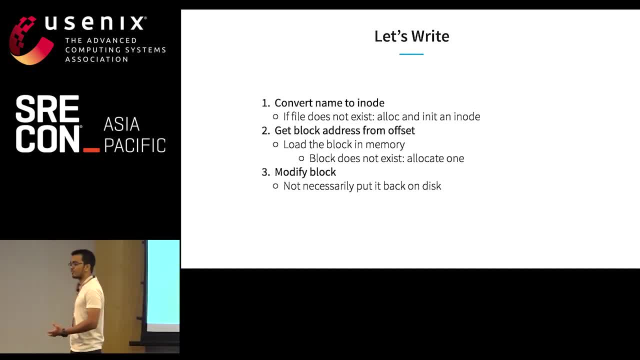 So you've written what you're going to do and while actually performing these three steps or whatever steps you're doing, if something goes wrong and if you come back up, then you actually know that what you're going to do, You actually know that what operations were going to be executed, and if you know those, 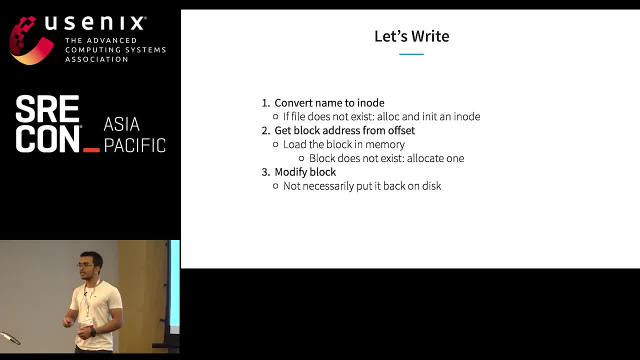 operations. you can roll back and come back to a consistent state. So that's what journaling is: You write what you're going to do and then do it. So then, in case something goes wrong, you can recover. Now there are some problems with this. 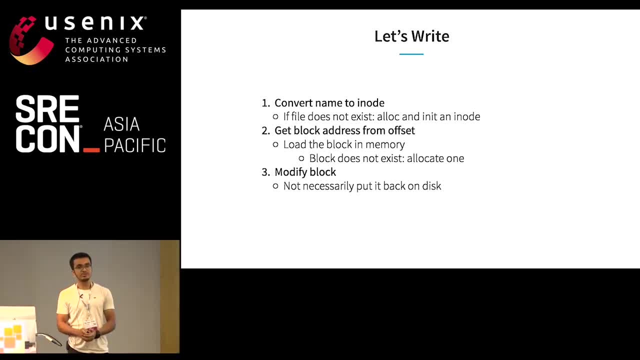 So, first being, you are writing contents to a disk. A disk is a device. A device can go wrong, go bad, and it's a single point of failure. Right, It is gone. Your data is gone. If, say, Thanos snaps his finger, half the storage devices of the world are supposed. 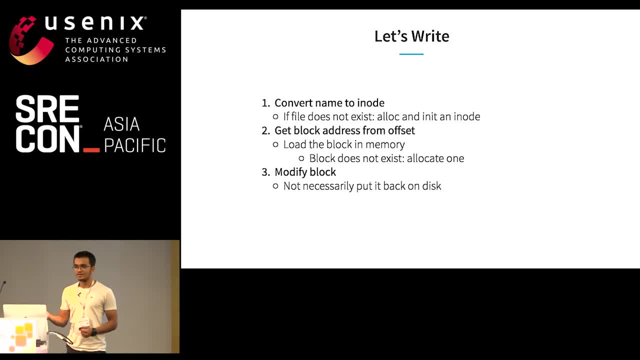 to disappear. What happens in that case? Fifty percent chances that your data will be gone. Single point: failure. Other being it's a physical device, so it can only read n number of reads bytes or it can only write n number of bytes per second. so if you have tons of CPU power and you want 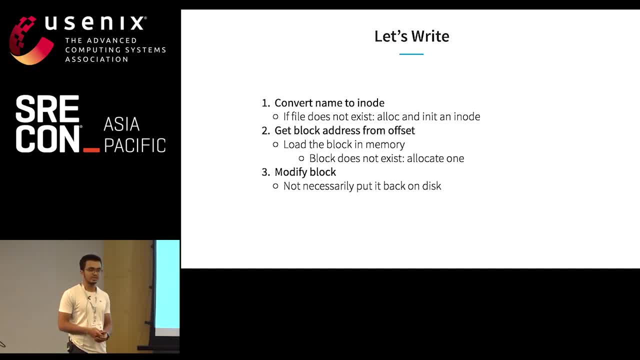 to do tons of processing from this data that is relying on the disk. disk will be a bottleneck issue because it has limits. And third being, again, it's a storage device and it's been manufactured and has storage capacity. that is fixed. So tomorrow, if you want more space, you cannot expand this because it's a piece of hardware. 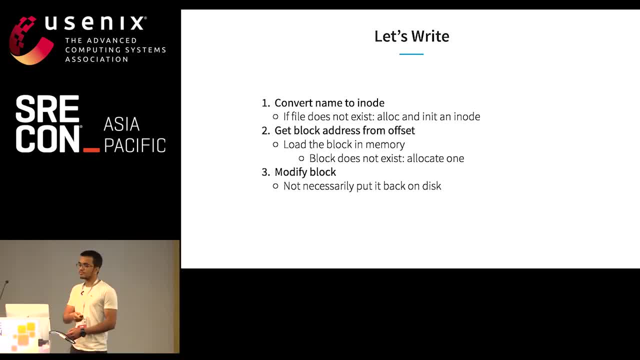 So these are some problems with it. Some of these can be overcome by using RAID. There is redundant array of disks, So still some problems associated like. it is presented as a single volume to your OS, so if your server or the host crashes, your single point of failure sort of problem. still, 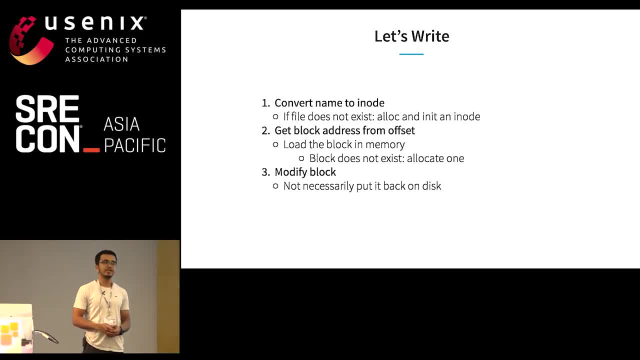 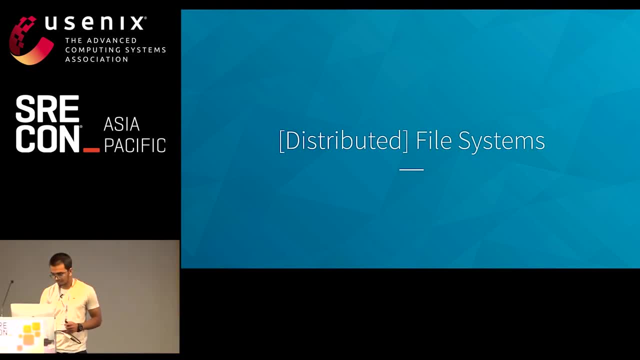 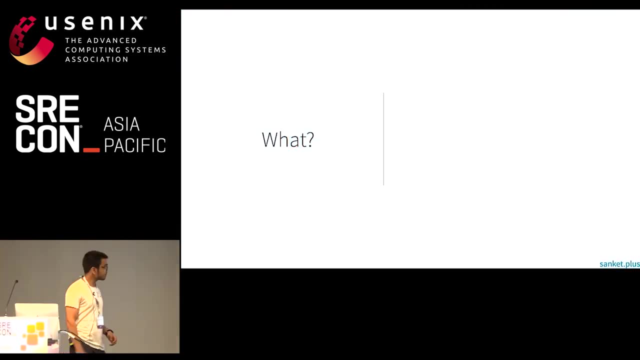 persists. So we won't be going into RAID configurations and we'll take a look at the next logical step that will overcome some of these problems called distributed file systems. Now, what is it? A file system, but distributed. Now you may ask: distributed, but distributed across what? 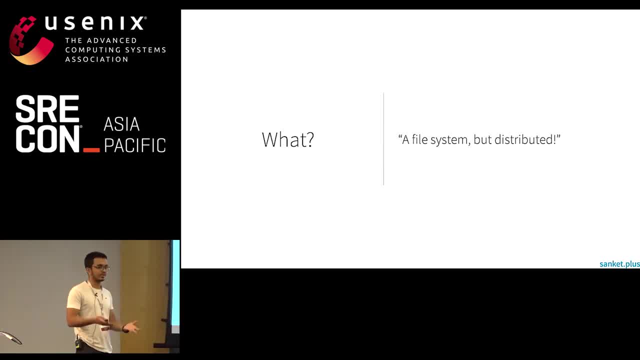 Across disks, across hosts, across data center, across geographies. In this case, it will be distributed across network of hosts. We'll see how does it look like, But why go distributed? Of course we want to avoid single point of failure. So if a host or a disk goes down your file system, your data should be still available. You should still be able to access it. You want to avoid bottleneck problems And of course you also want to scale your storage space. You don't know, because data size is ever increasing, so you don't want to be bound. 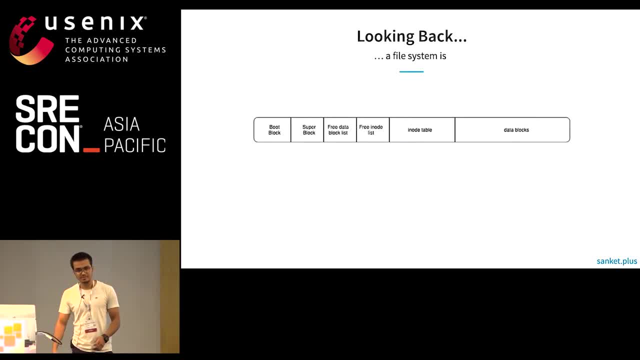 by your storage space. Now let's take a moment. look back what our file system looked like. It was made of metadata and data to classify it on a really high level. So all the inode table, free inode list, super block- all this was metadata and the data part. 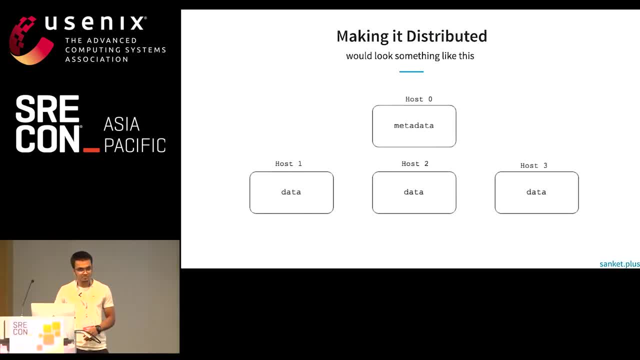 Now let's try to make it distributed. So let's take metadata, put it on one host. Let's take data, put it on several hosts. There you go, your file system is distributed. Now you may not sound convinced, but let's try to see the files that we saw it in our normal file system. example. 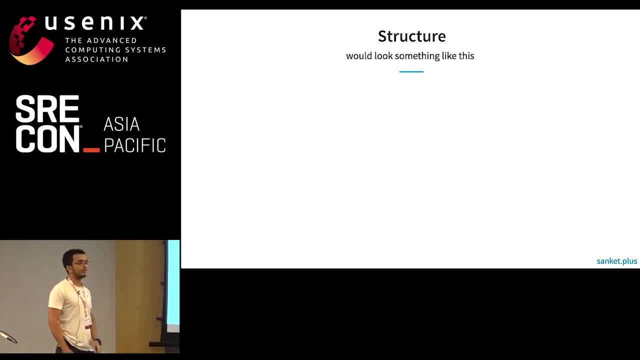 slash, etc. slash password. Let's see how does it look like in our distributed file system. So host zero is metadata host. What kind of metadata file will have? File will be divided into blocks and blocks will be placed somewhere. So in our earlier case there was only one copy of the block in data blocks list. 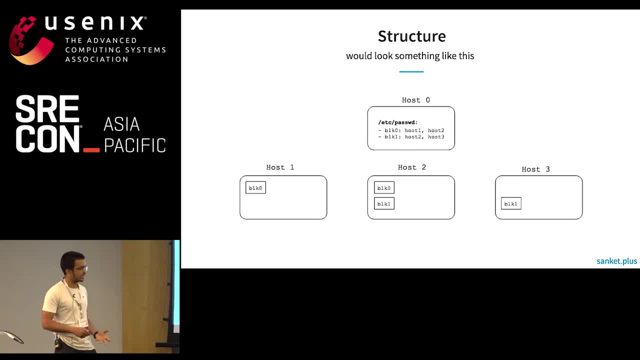 Now, because you're making distributed, you want to tolerate failures, You'll be creating multiple copies. So say, etc. password was divided into two blocks, block zero and block one- And here we have chosen to create two copies. So block zero is placed on host one and two, and block one is placed on host two and three. 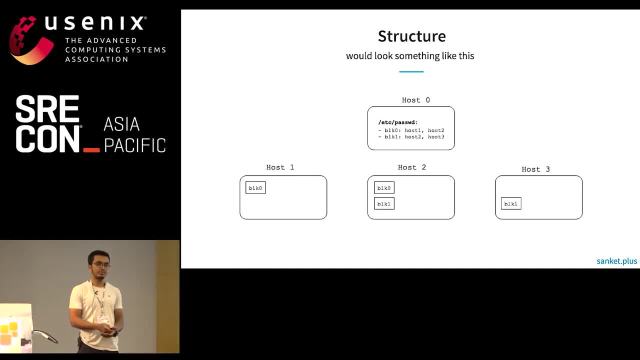 Of course, this is configurable. We've created two copies for now. Now this is what it will look like in our distributed environment. Now let's see: how does it solve our problems? So the first problem we talked about was a single point failure. 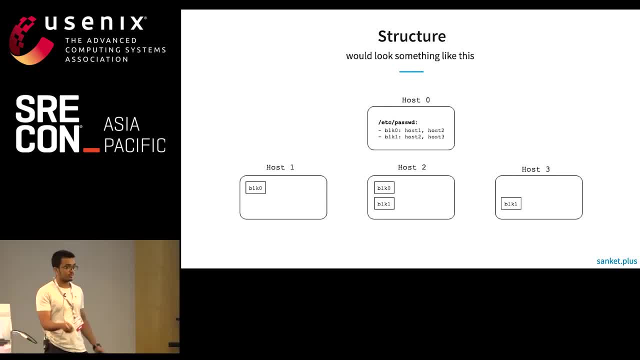 How is it solved? Because we have two copies or multiple copies. Say, host one went down, Block zero. first copy of block zero is not available, but it's still there on host two. So this is how that part is solved: single point failure. 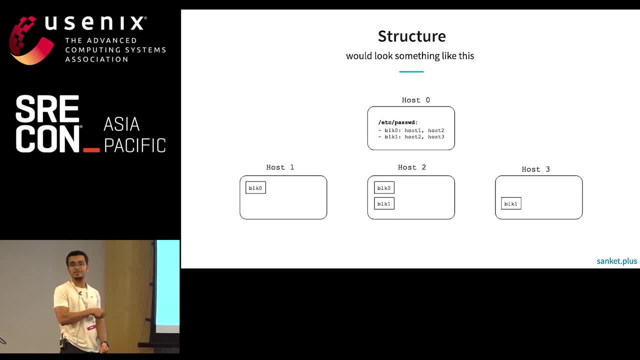 Now you may ask that there's only one copy of metadata. So what if this thing goes down? You're out in the water, right? We'll see how different file system handles this single point- failure of metadata part. But at least for data part you're sorted. There is no single point failure anymore. You've got multiple copies. The other problem was bottleneck issues. Now you've got two copies. So if somebody wanted to read etc. password file, they've got multiple options to go to. So this really helps. 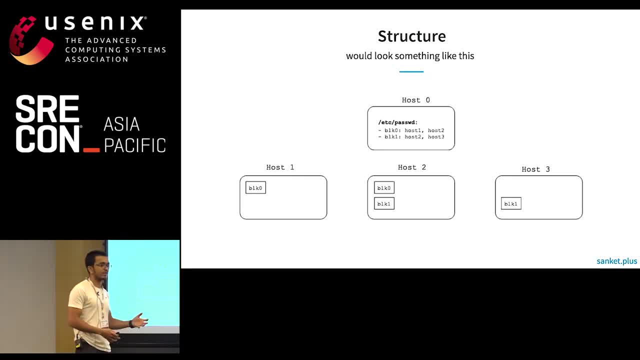 Let's take an example. We had a data set. We had a data set of LinkedIn's member data, So it will be a sort of a table And tons of queries- business intelligence queries- will be needing access to this data set to join some other tables. 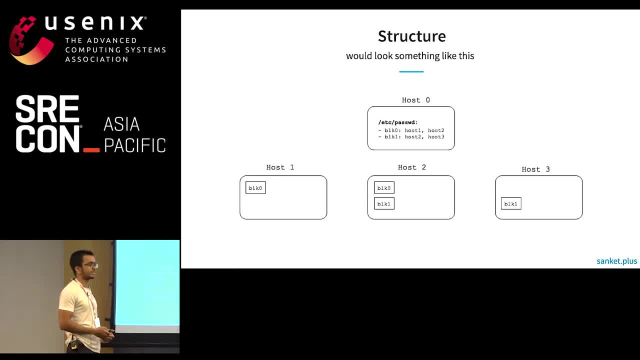 So these are really demanding data set- LinkedIn's member data set. So what you can do in that case is, for that file, you can increase the replication factor. Instead of creating two copies, you create ten copies, for example. So each block of the file will be available on ten different hosts. 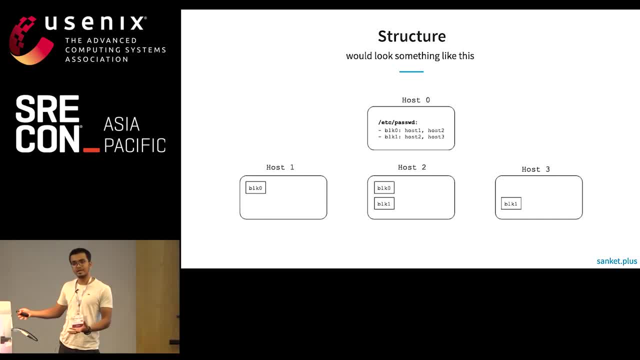 Now ten different hosts will have their own independent bandwidth. So now, instead of in case of a normal file system, you've got ten times more bandwidth in this case. So if users are running queries that are distributed across ten hosts, then you've got ten times more bandwidth. 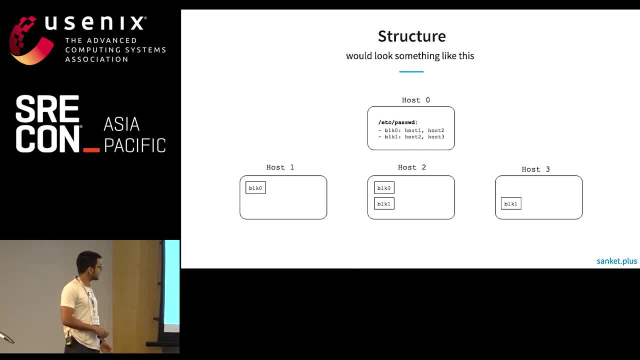 So there you go, You solved your bottleneck problems, And the last problem that we discussed was storage space. That storage space, Storage is not scalable. So in this case you can always go on and add one more host, say host four, host five, and your storage space will scale. 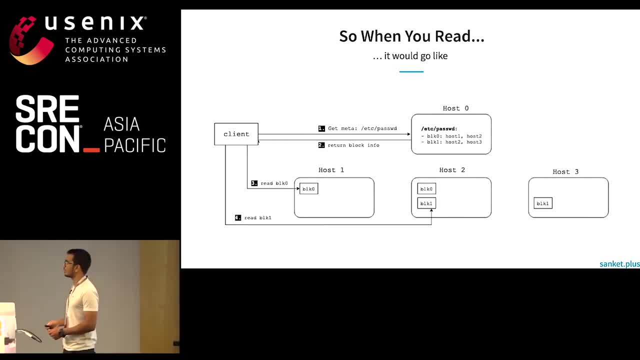 Now let's try to read Same file. You've got someone who wants to read. Metadata is located on metadata host, So here's what you will do. First, client will go to metadata host. It will tell that I want to read this file. 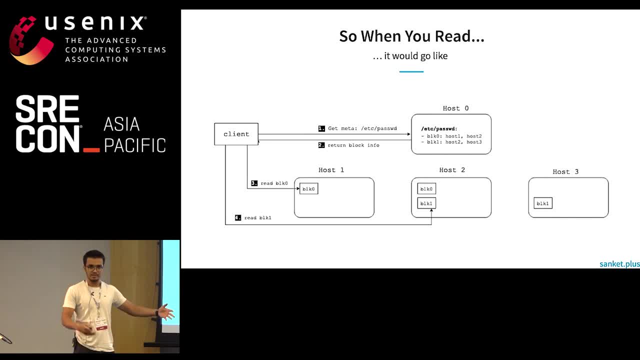 What metadata host will tell is: these are the blocks And this is where they are located. So now what client will do is it will go directly to the host that contains those blocks And it can try to read. So you can see that it is only connected. 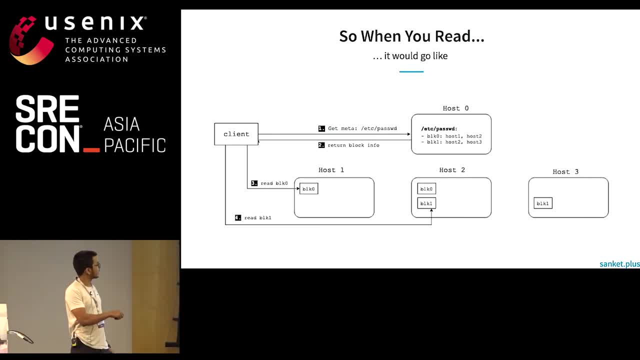 The metadata host is connected only once And now the client can go directly to the host that contains the blocks, actual blocks- and go read the blocks. If it wants to read block one, it can go host two. Now in case host one was down. if it's down for some reason, 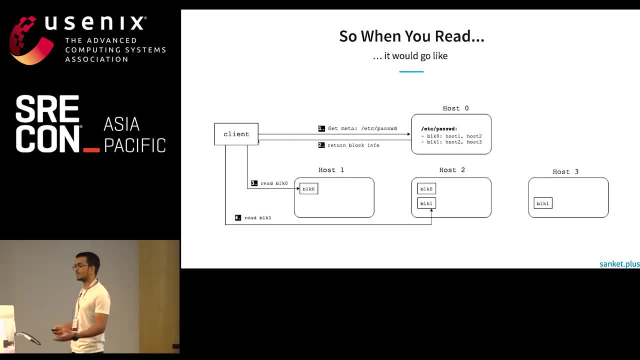 your client knows that. where else to find block zero? So if host one is down it can go to host two. Similarly for block one. Now you can see a potential bottleneck here, because to read or write every file you need to go to metadata host. 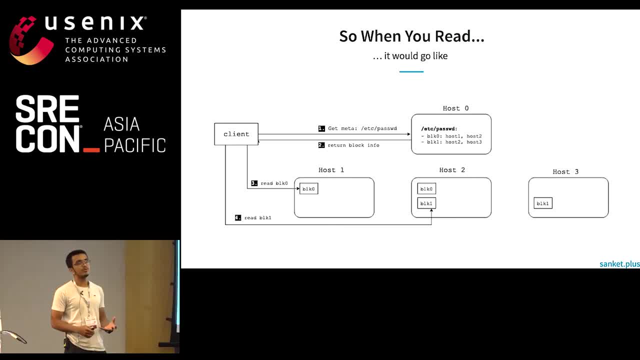 So this can be a potential bottleneck. But in most cases all this metadata is kept in memory, So it doesn't take much of computation power for master. So at a very later point of time when it starts to become a bottleneck issue, 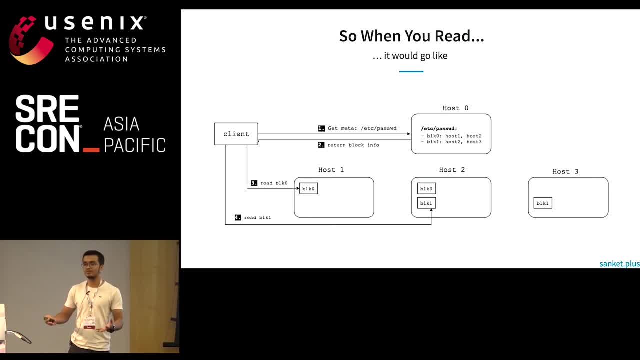 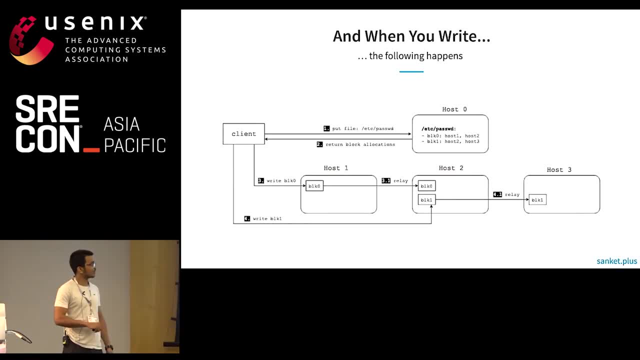 there are some ways to sort it So you can have two metadata nodes and they distribute the metadata amongst them. Now what if you want to write a file- Well, somewhat similar, You'll first go to metadata node. You'll tell that I want to write this file. 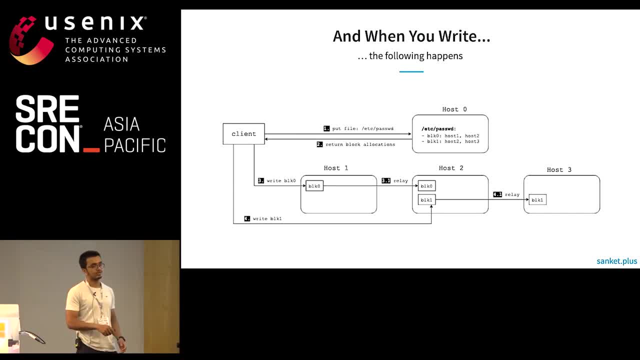 What metadata node will do for you is it will divide you into blocks And it will also tell you that this is where the blocks are supposed to go. So it'll do the allocation part, basically, And tell client the allocation. Now client will go and directly write those blocks to the data hosts. 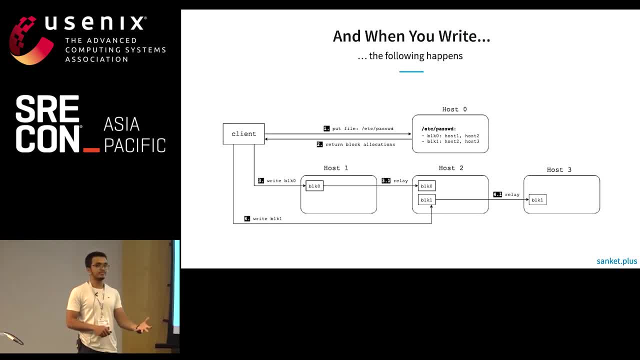 Now, while writing, just to optimize things a bit, what you can also do is you can relay the block to the next host So that in parallel you are writing it to two hosts. But this is just an approach that HDFS seems to be doing. 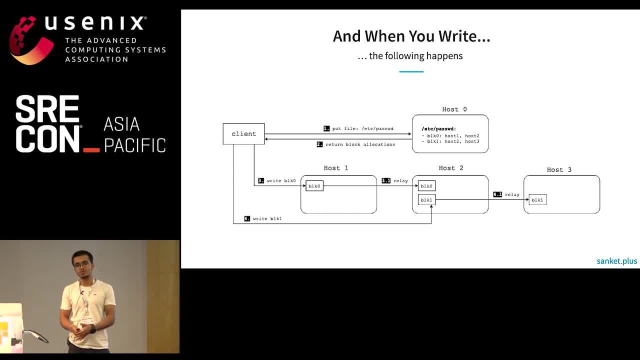 You can always write one block. Say, you're writing block zero on host one. When you're done, you can go and write on host two. It's up to you. So this is how a write will look like. Now let's try to see it in action. 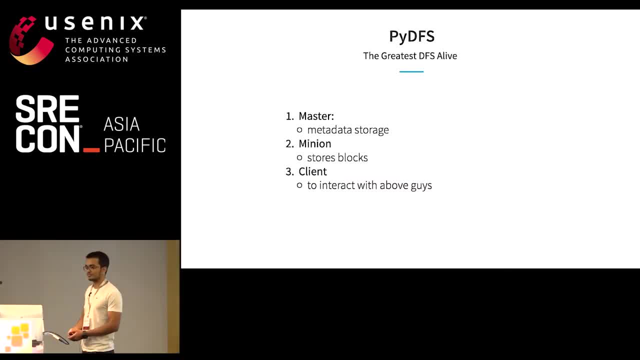 We said that we made a cute little distributed file system. Let me introduce you PyDFS. These are the three components that we'll be dividing it into. We have metadata storage- Let's call it a master. We got data host- Let's call them minions. 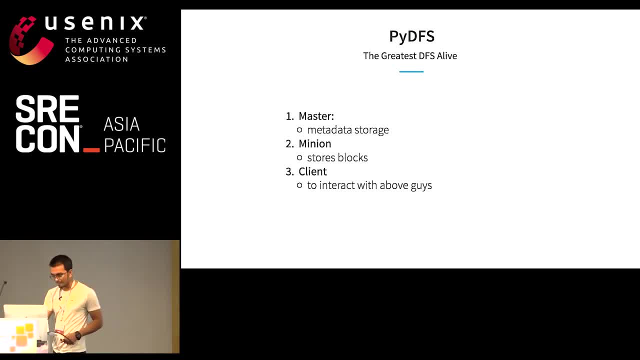 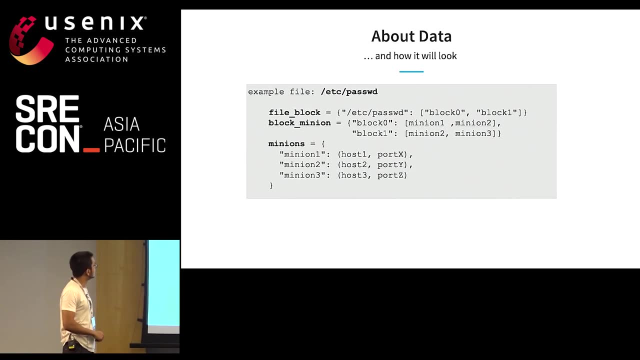 And, of course, we'll have clients to interact with these, These two. Now how will the file that we've been talking about, slash ct, slash password, will look like in this case. This is the file. We'll have a dictionary of file to block mapping. 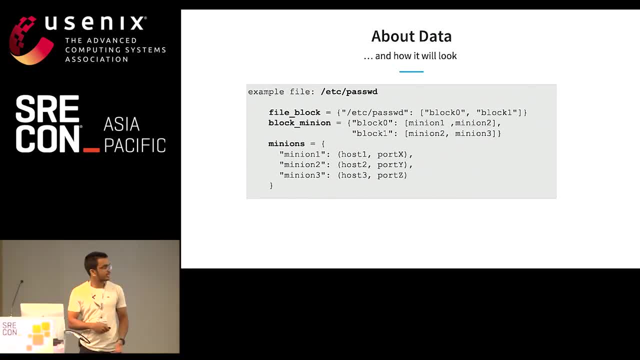 That is, a file is divided into all blocks, That, in this case, block zero, block one. We'll be having additional dictionary that will track the blocks allocation That where each block is located at. So that will be a block to list mapping. 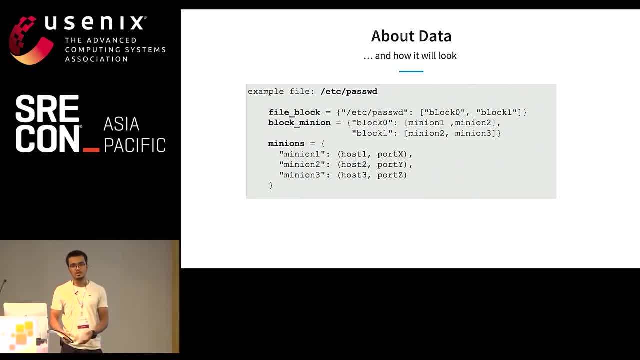 And then we'll have a list of minions, That what all are our data hosts. There will be some more properties, The first being replication factor. So far, in the examples we've been seeing, we've been creating two copies of each block. 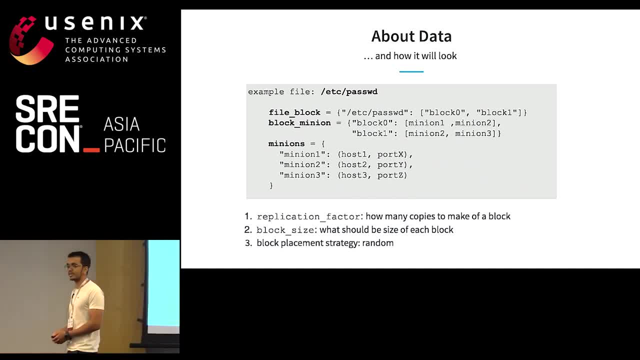 But this really is configurable. Say, we discussed, like in the LinkedIn members data set case, we want to increase the replication factor. It makes sense, So that will be one of the properties, That- how many copies of the blocks to create? 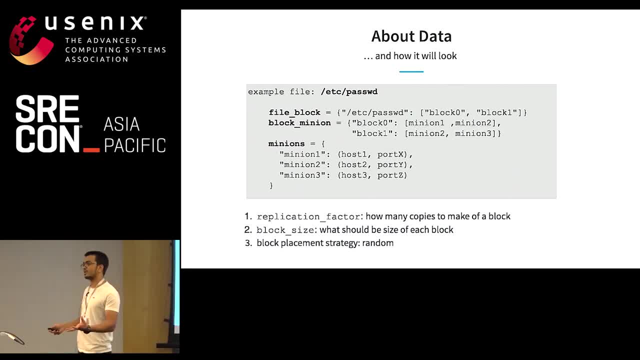 Other will be block size. So we had a block in our typical file system as well. We have blocks in here as well. But what really different here is? in case of typical file system the block size are usually half a kilobyte to four kilobytes. 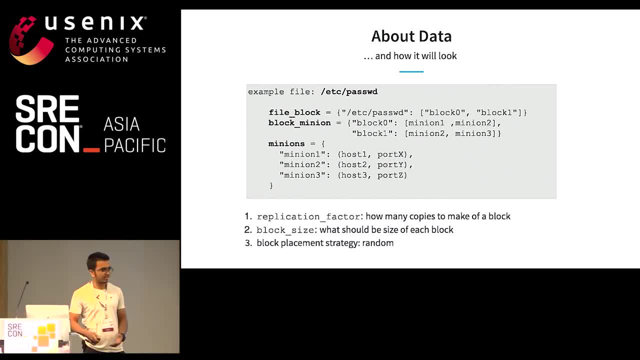 So this is the block size that is used in our normal file system. But in this case, because you have a really huge storage space and huge data sets, you generally increase the block size to 64 MB or 128 MB, So that will be block size. 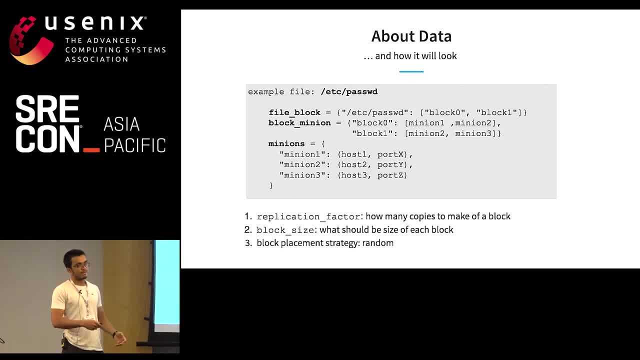 And, of course, the block placement strategy. So metadata node does the allocation. In this case, master will be doing allocation, that where each block should be placed. In this implementation, our tiny implementation, it will be random, But in real world you will be using some heuristic or logic. 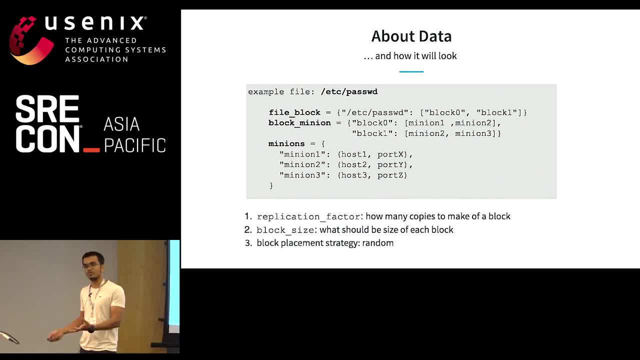 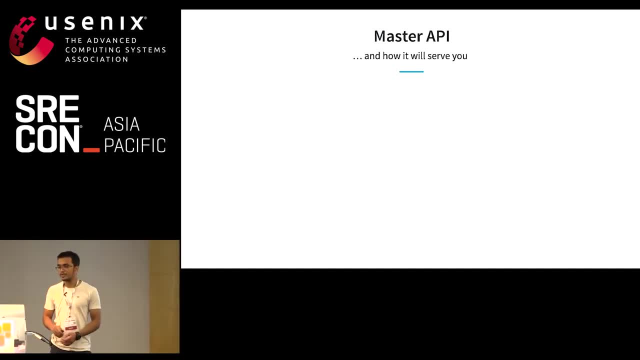 to decide the block placement, Like where all the blocks should be going, On what data host your blocks should be going. You want to use some logic. after that, Let's take a look at the API. How will it look like? Master will have two functions. 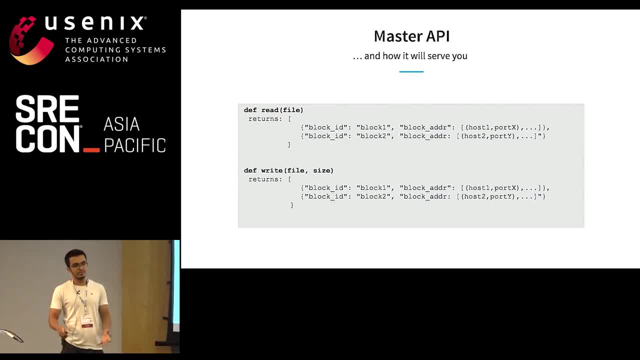 Read and write. Read: you just give a file And what it returns? Fantastic blocks and it will find them. That is list of blocks and where are they located. In case of write along with the file, it will take size. 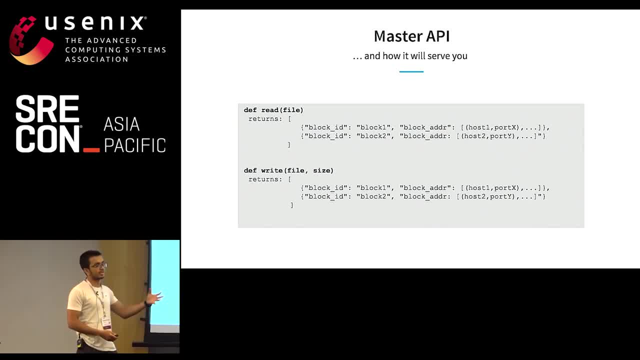 Why size? Because what master does is, given a file, it will divide it into blocks And those blocks has to be placed somewhere. So to divide it into blocks it needs size. So you give a size as well. It will do the allocation using whatever logic it uses. 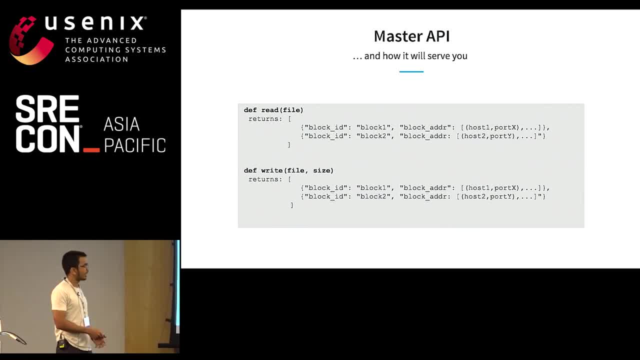 In this case it happens to be random And response would be somewhat similar. How will the minions API will look like? Well, minions will be relatively simple. After all, they deal with these blocks. So, given a file, it will divide it into blocks. 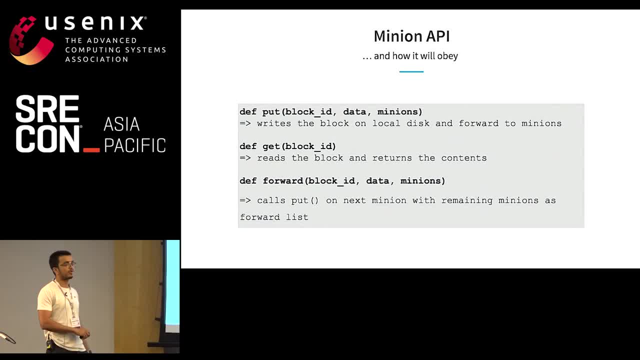 So given a block. if you say get me this block, it can just read block from its local storage and get it back to you. If you tell it to put, it will put the block on your local disk And it can also forward it to the other minions. 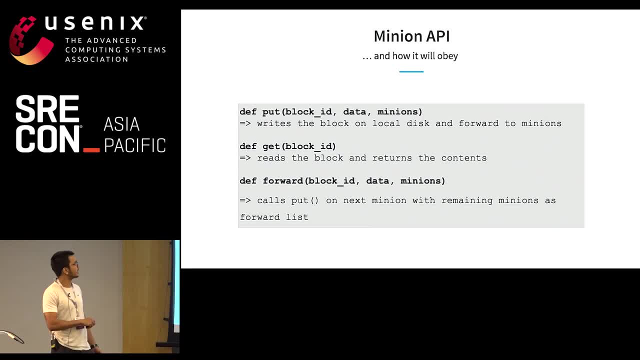 like we just saw in the diagram. So if you call it put on a minion, it will write the block on the local disk and it will call put on the next set of minions that are in pipeline. Now how will they communicate? So obvious choice would. 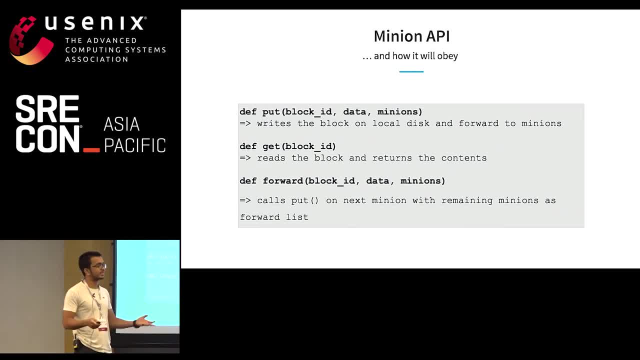 like. the natural choice that would come first to your mind would be an HTTP API. Like clients, minions, masters will be communicating over HTTP protocol. In this case, we'll be using RPC remote procedure calls. Why No particular reasons, But the seems to be using RPC. 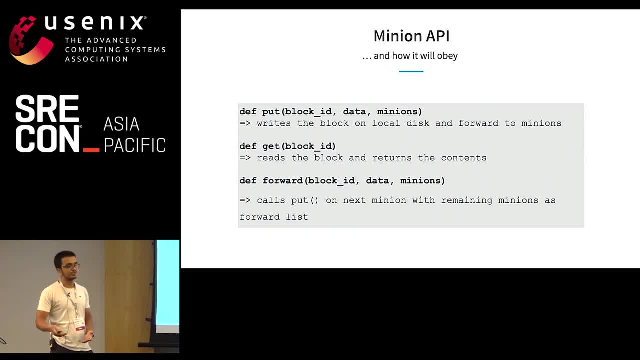 because after some point of time it makes sense to use custom procedure calls protocols. So that is why we have chosen to use RPC. here. We'll be using a mobile protocol. What do you call RPC? Let's also take a look at some code. 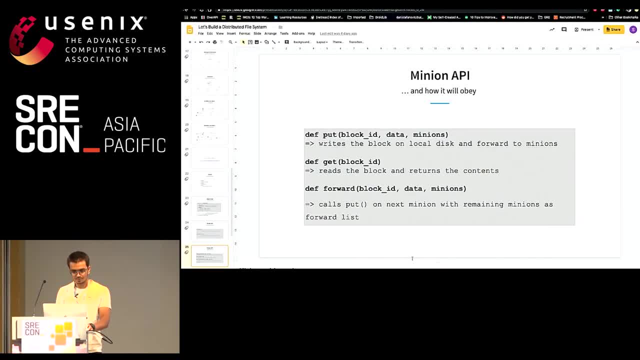 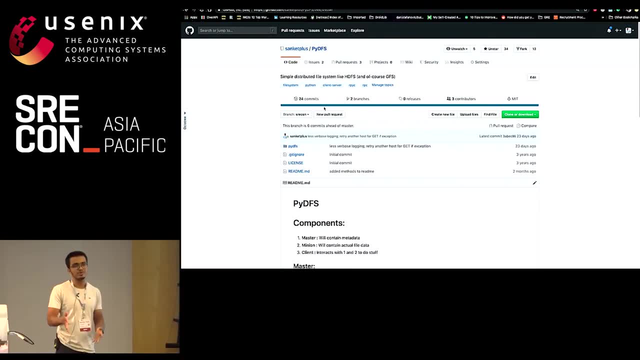 so that it makes sense. It is there on the GitHub repo. The code is really simple. It should be approximately 200 lines, So you can go home and check it out. My username is Sankitplus. Repo is called PIDFS. 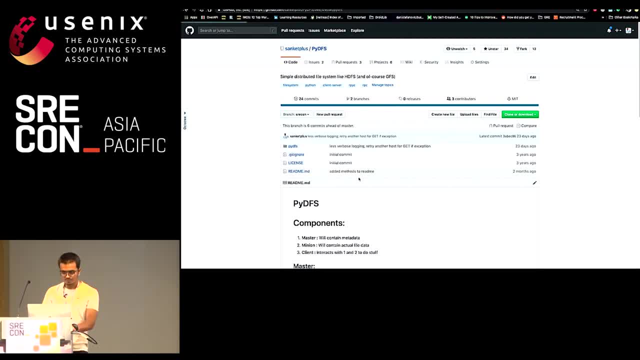 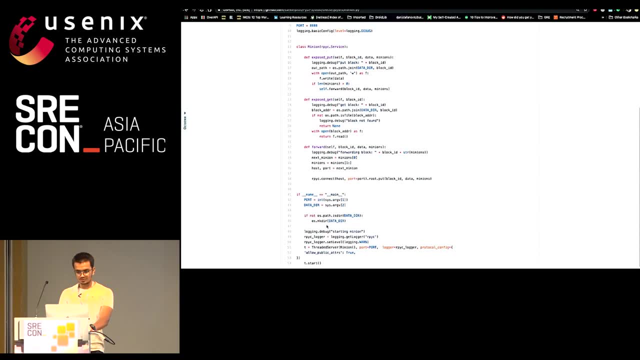 And code should be under srecon branch. Let's take a look at minions first. This should be relatively simple. So this is where you start the RPC server, so that you can remotely call the objects of, say, if the client, if it is a minion. 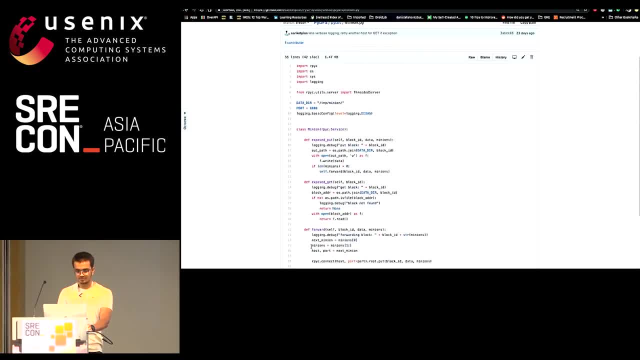 then it can call other minions, put. So here we just start the server. This is the class minion. So you have put. Put will take block ID, It will take data And it will take list of minions. What it will first do is it will write it on a local disk. 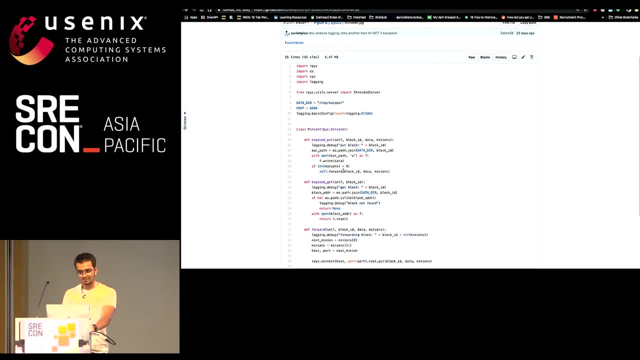 whatever the block you've given, And it will call forward. What forward will do? It will connect to the remote minion. So these are the RPC calls And it will just call: put on that minion. If you want to get a block, you just give a block ID. 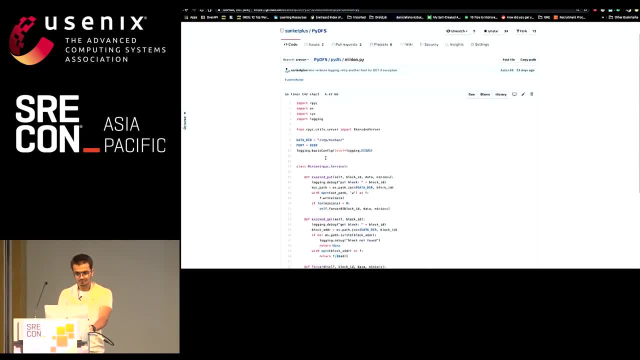 It will read from the file and return it to you. That simple. If we quickly take a look at master code. these are the data sets that we talked about: File to block mapping, block to minion mapping and, of course, the list of minions. 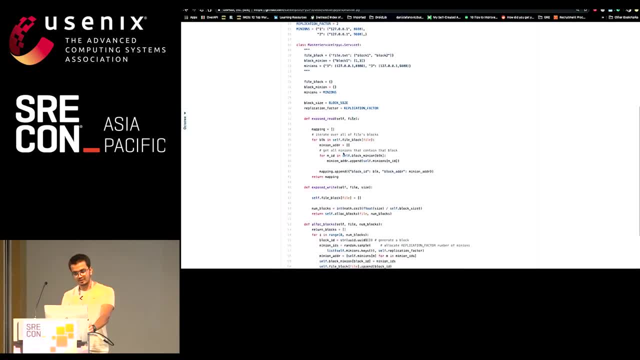 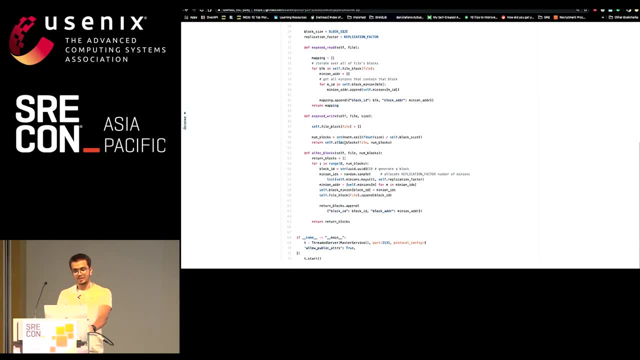 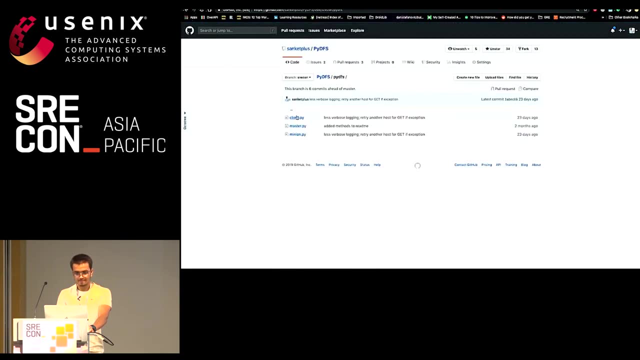 You've got a read, You just give it a file. It will return you the mapping Blocks to where to find the mapping. If you call a write, it will allocate blocks And it will read on the allocation Client. client will be communicating with these two. 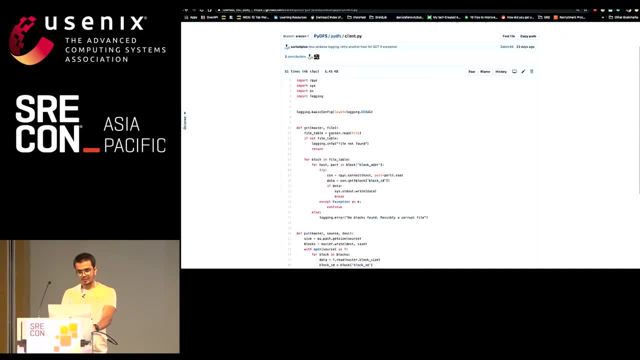 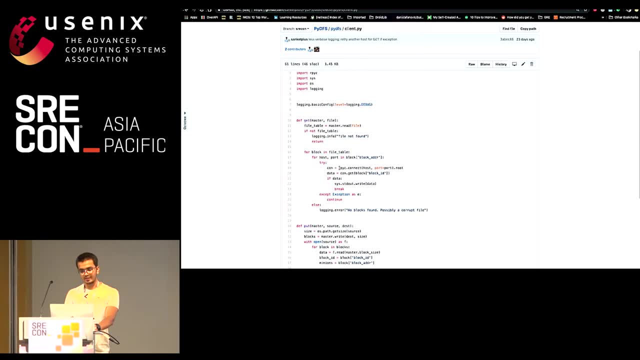 as we saw in the diagrams. So if you call a get, it will call a read on master because it needs to get the metadata, And for each block it will be connecting to a minion and calling a get on minions. Similarly it will be for puts. 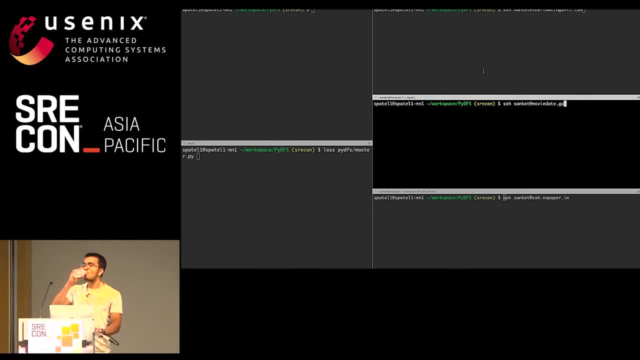 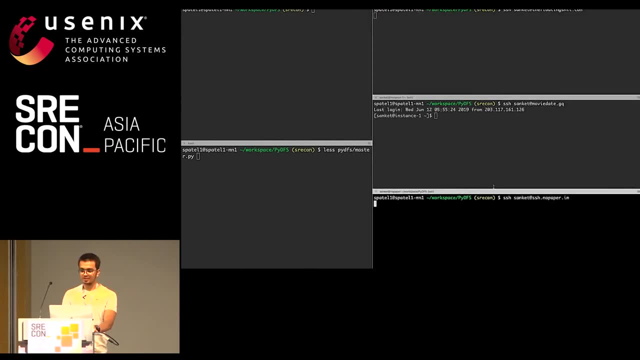 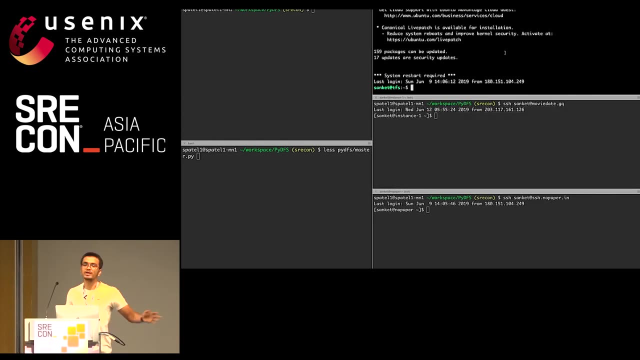 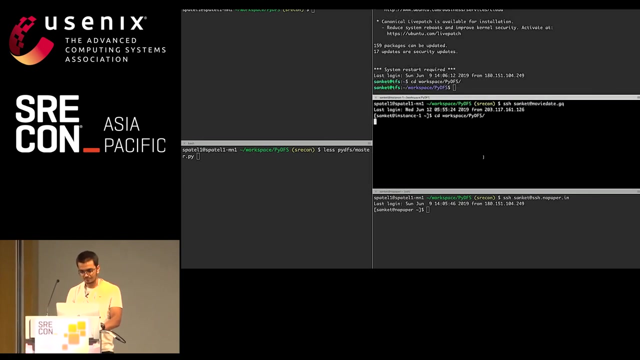 Now let's try to see this in action. So we'll be starting up three minions. These are three actual cloud hosts: Two are on Azure Cloud, One is on Google Cloud, just to get the feel of distributed file systems. We'll start the minions. 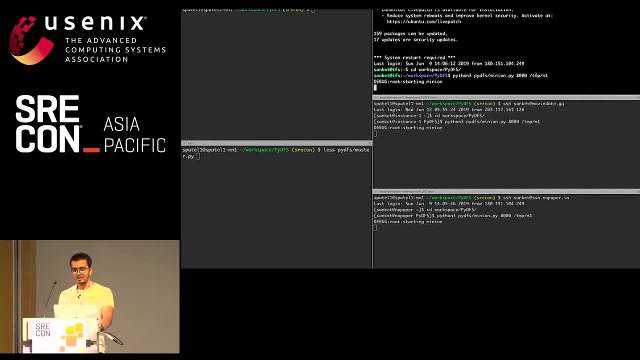 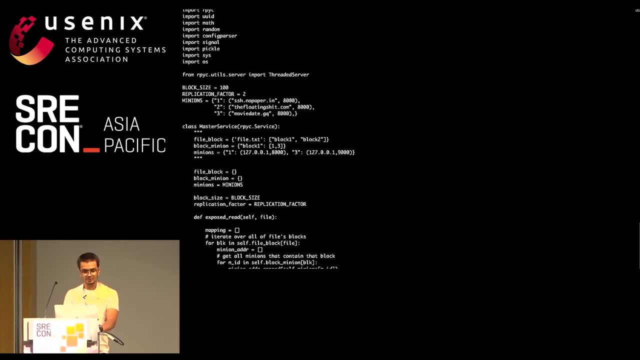 So the parameters that we're giving is the port that it will be listening to and a directory where the blocks will be written. This is our master. So, as you can see, we have three minions that are really distributed across the internet. Replication factor we are setting is two. 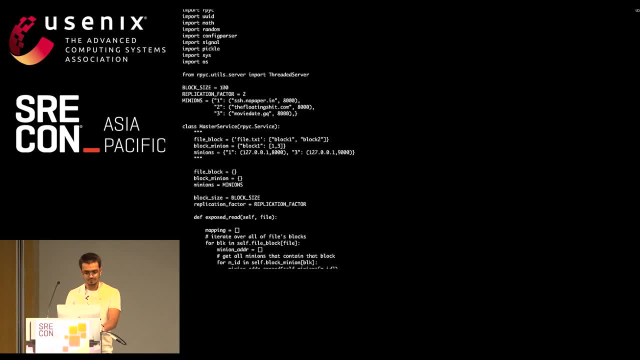 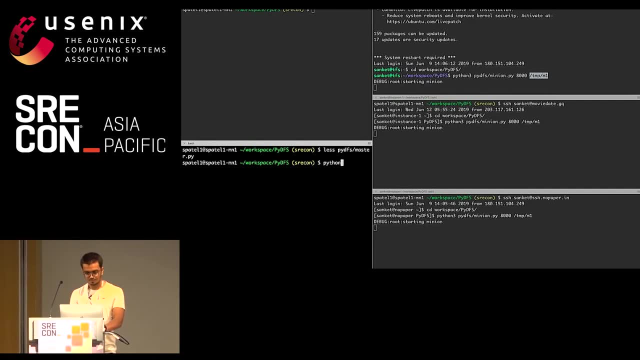 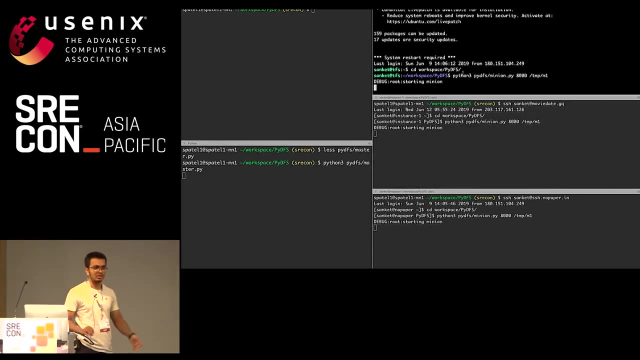 And block size is 100.. Just for this example, Let's start the master as well. So we have master running on our local machine. We got minions running across the distributed server somewhere on the internet. Now let's try to put a file. 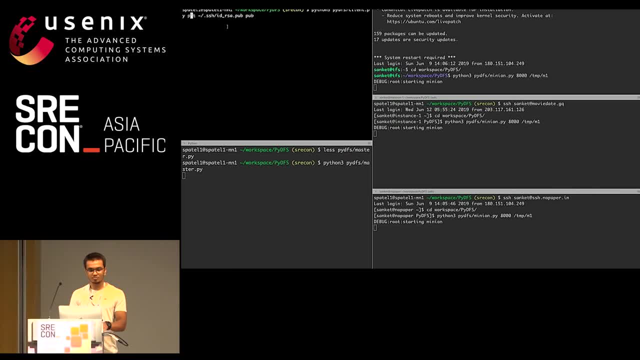 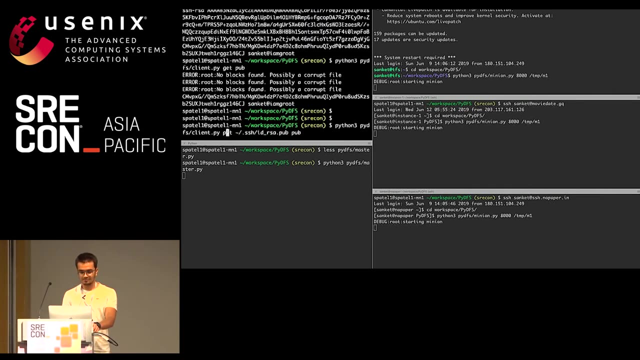 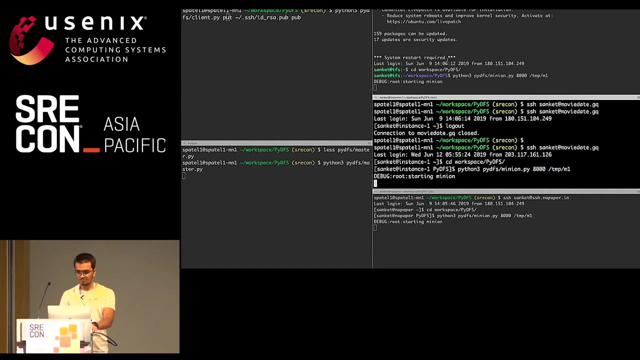 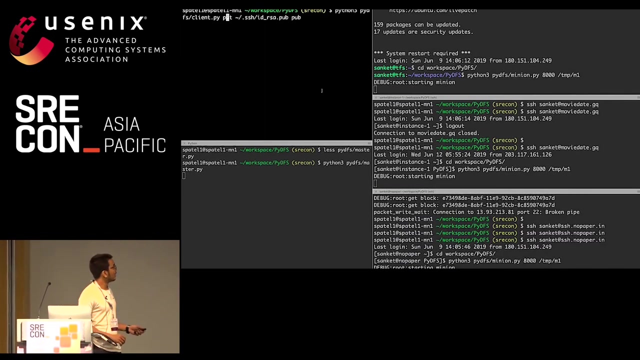 So we call a client, We say put, I'll be putting my public key And we'll be calling it pub. I hope this is readable. Or should I zoom in? Let me So. when I call a client, when I will call a put. 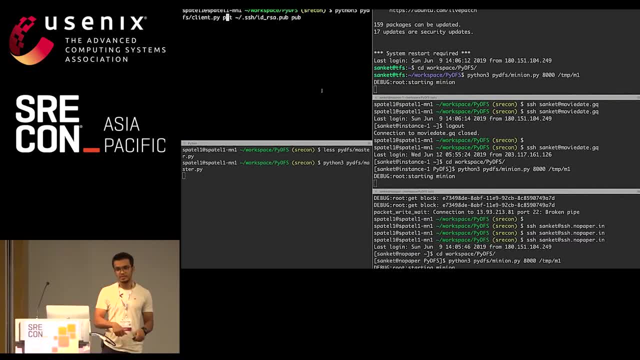 what client will do it? it will first go to the master that is running locally. Master will do some allocation And whatever the allocations are done, it will call put on minions that are on some remote hosts. So let's try to see. 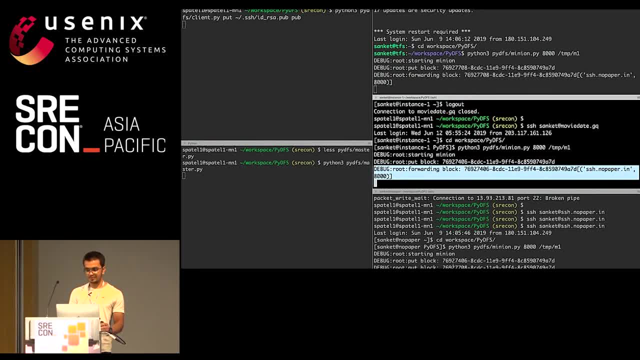 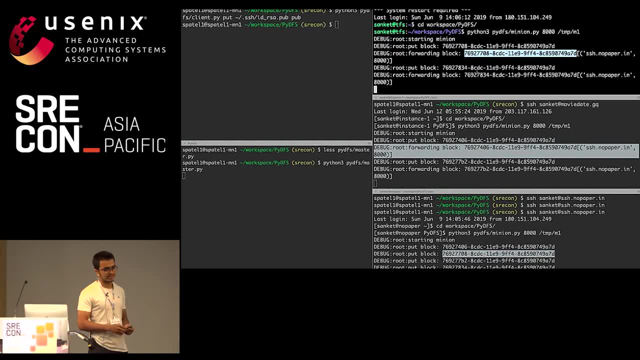 So, as you can see, put block has come. It is forwarding block to some other server Here. put block has come, So randomly. blocks are getting distributed across hosts because that's what our strategy was: We'll be placing blocks randomly. So our file has been written. 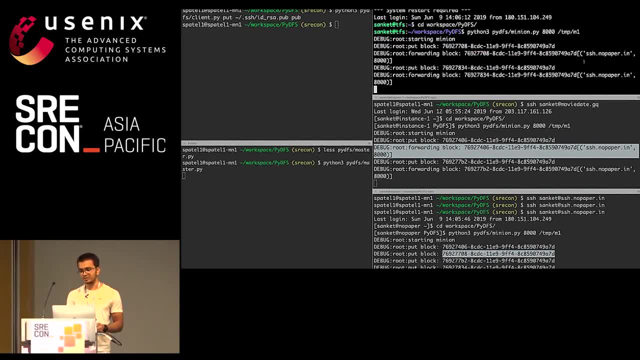 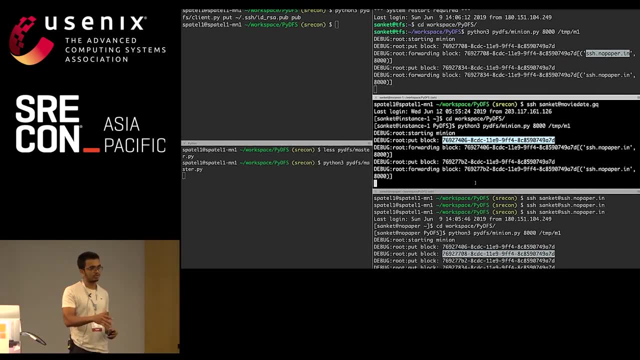 Some blocks are on this server. It has been replicated to this server, Some are on this, So they are basically distributed. So you put a file, Your file was divided into blocks of 100 bytes And all the blocks are put randomly on some servers on the internet. 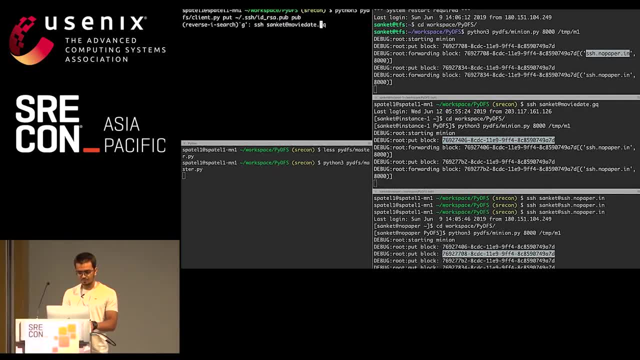 Now, if you were to read this file, we'll call get. We'll say we want to read the pop file. That's what we put the name as. So similar workflow will happen. It will go to our master that is running locally. 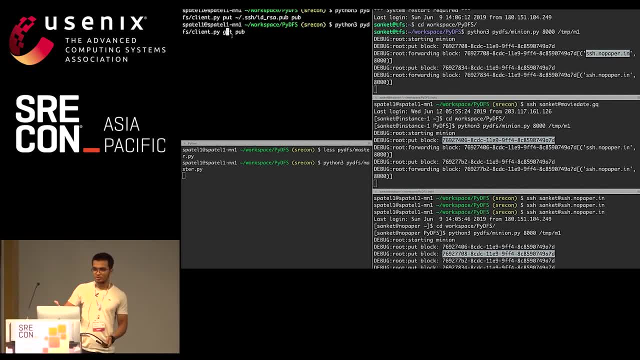 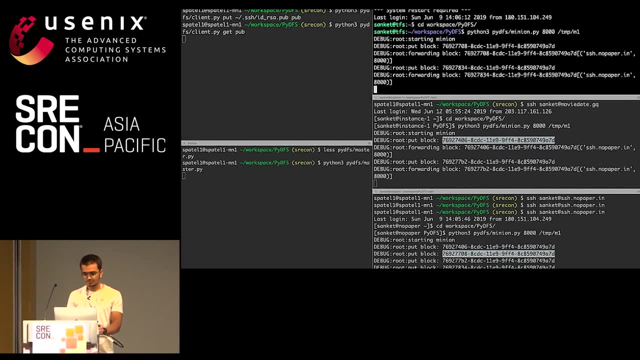 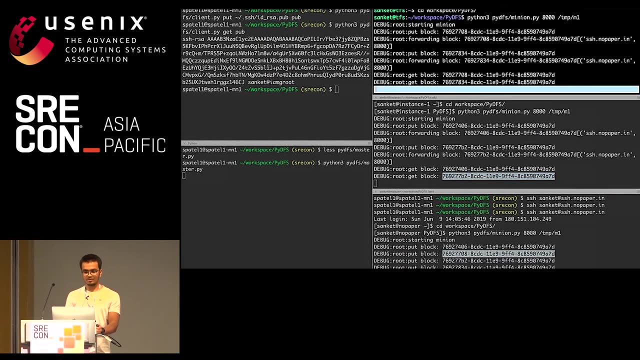 Master will tell that these are the blocks. These are the two of the three servers where they are located And our clients will be contacting those minions. So you see, get block has come, Get block has come, One more get block, And there you go. 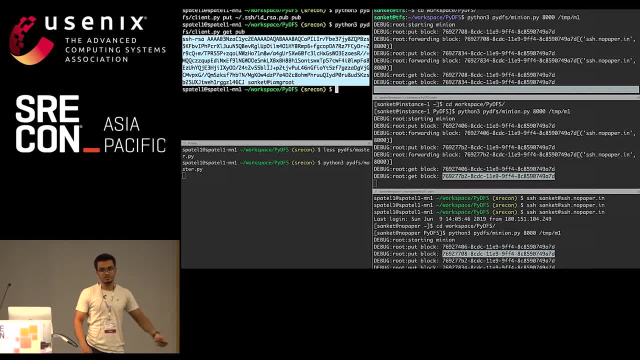 The file is read from across the distributed hosts And it's been presented to you Now. one of the reasons we went distributed was you can tolerate node failures. So what if one of the minions went down? Let's try to see what will happen. 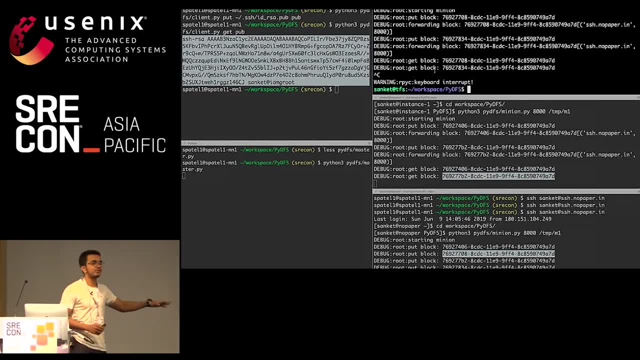 So we stop one minion. So all those data blocks that were stored on that minion are not available because the server is down. minion is down. something happened Because we went distributed. we made two copies. Your data should still be available. Let's see if it is available. 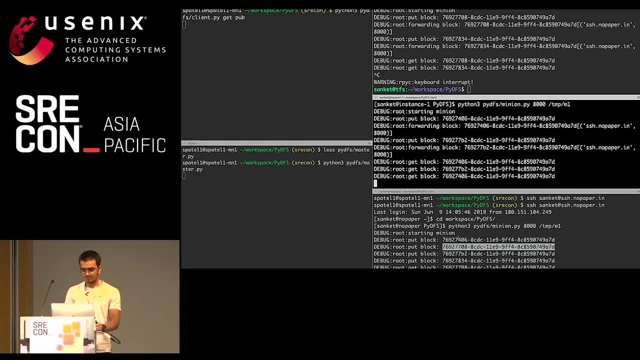 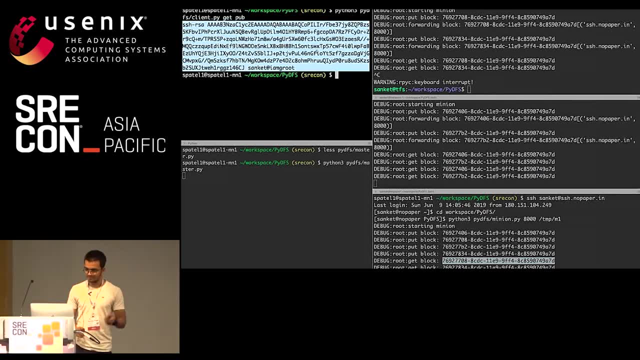 We'll call get again. Now see the queries are coming on third minion And you still have your file available. So this is one of the reasons why you go distributed. Now what if one more minion went down? Your file might go unavailable because you created two copies and two minions are down. 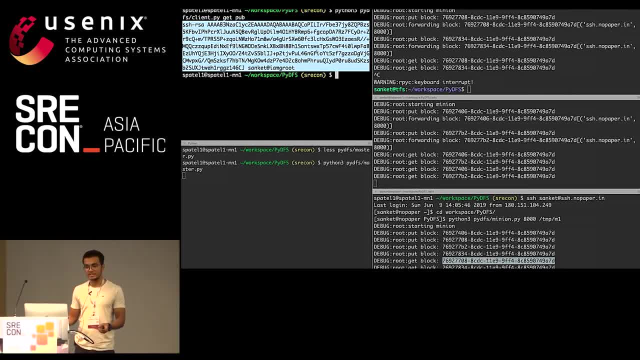 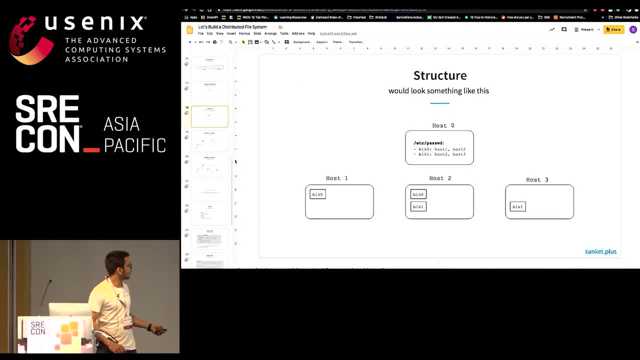 So there are chances that your file is not available anymore. While I'm saying chances, let's see A case can happen. where, say you had your blocks distributed like this: host one went down, host three went down, two hosts went down. 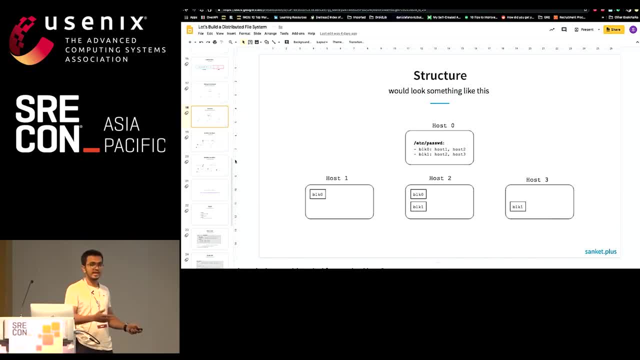 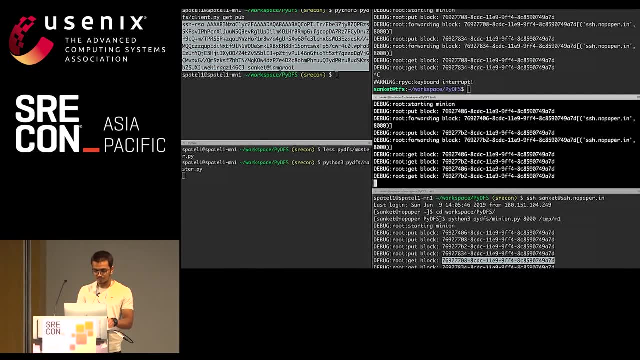 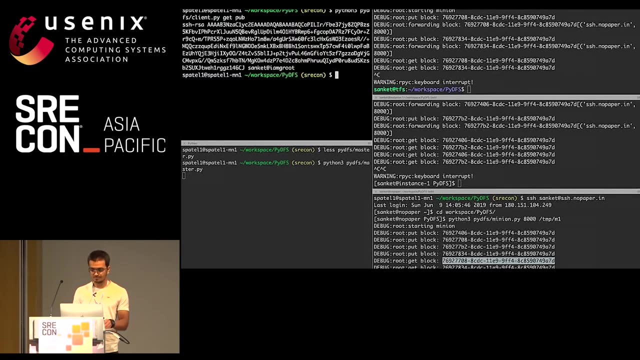 but you still got both the copies available. So this can happen. But if host two went down and three went down, you got block one is missing. So let's try to kill one more and see what happens. Two minions down. Let's try to read the file. 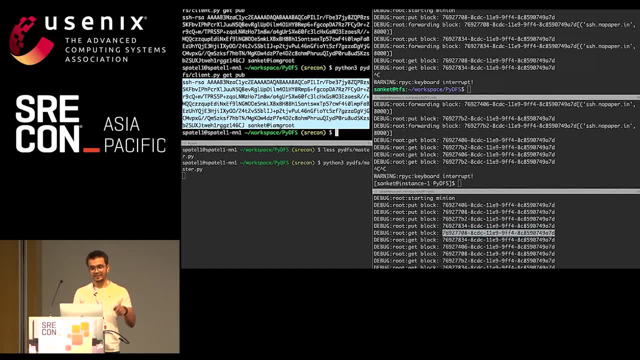 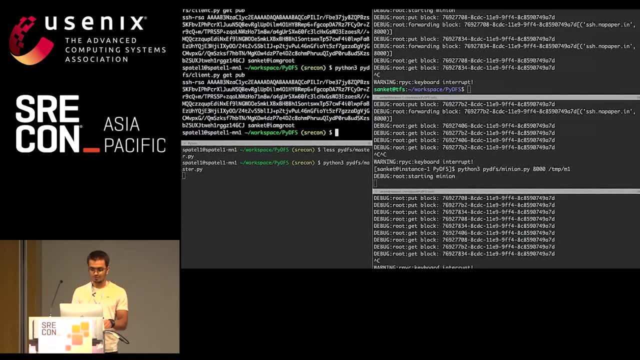 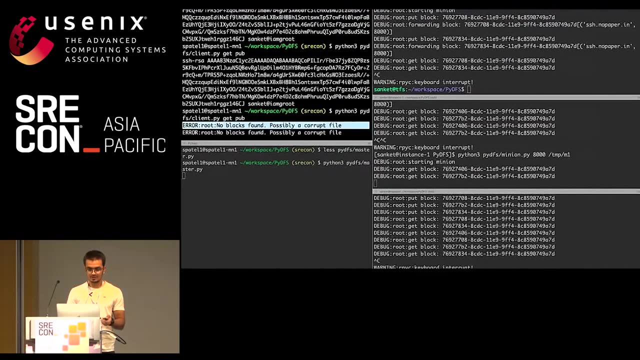 OK, it's still available. So it was the case that we described. So we'll do the other way. We'll start this one and kill this one. Now it should go corrupt. No blocks form. possibly a corrupt file: See no blocks form. 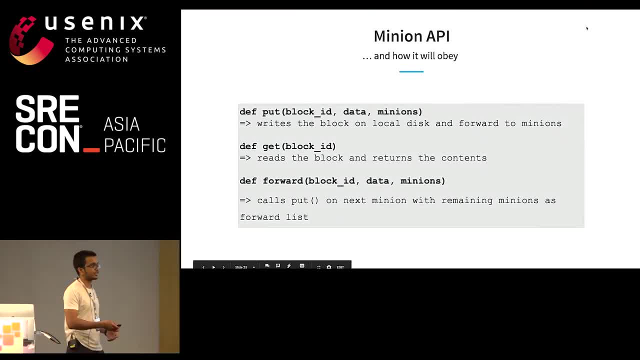 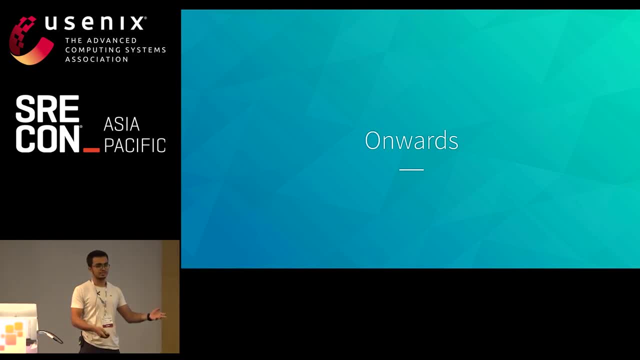 So this is what it will look like in actual distributed environment. This is how the reads and writes will go. Now where can you go from here? So this is just a toy file system. You cannot, of course, use it. It's not production usable or anything. 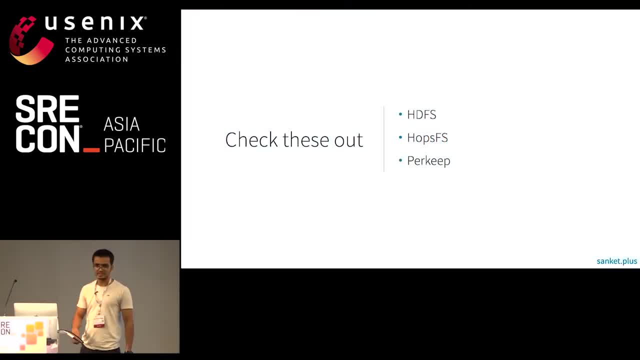 Just to understand the concept, we used it, But these are some of the existing file systems that the world uses, The most widely used or the most famous one being HDFS. That is Hadoop's database, Hadoop's distributed file system. 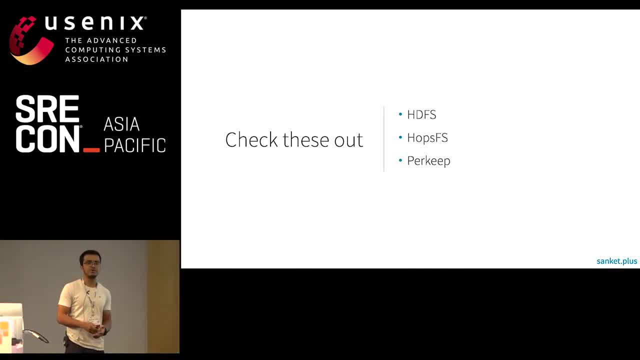 There's also HopsFS. that was created at Spotify. There's a bit of modification on HDFS- You can see what they do differently- And there's also Perkip. What Perkip does is it's a storage for your personal data. 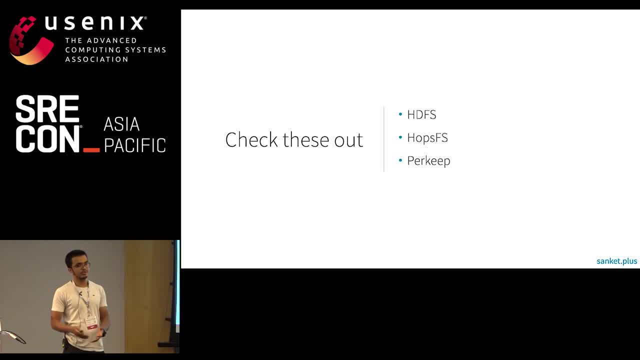 It can be replicated across storage providers like Google Drive S3, Azure Cloud Storage. So these are some of the distributed file systems that are out there that you can check out. Now, not everything science is gold, So in this case it sounds all good and all well. 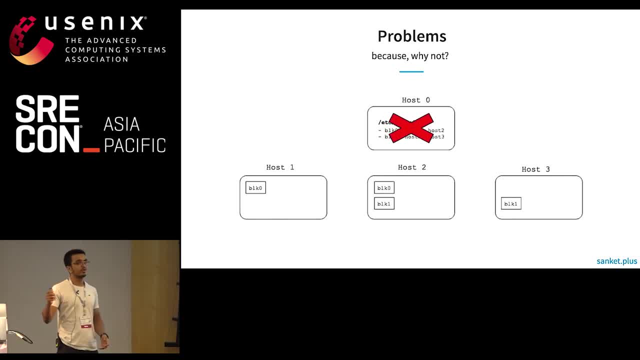 but things can go wrong here as well. What can go wrong? We initially said that what if we had only one copy of metadata? So what if metadata goes down? So let's see how does this file system handle? because we've mentioned them. 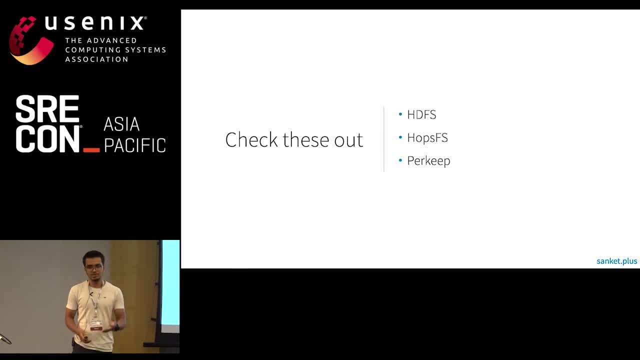 So in HDFS, in real normal basic operations, your metadata is stored on a disk, local disk. So because it's a disk, it's a single point of failure. we talked about it. So what it can additionally do is, while writing it to a local disk, 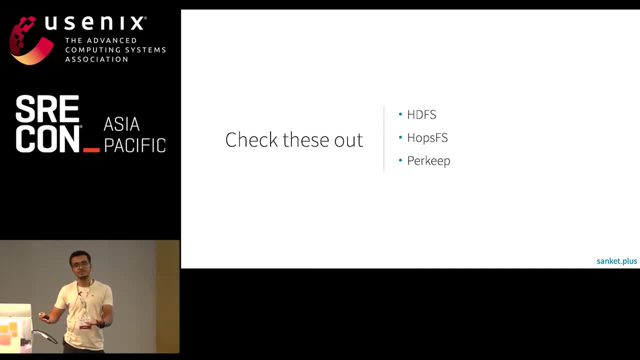 it can write it to a network disk. So there you go, You've got two copies. You still have one master process of the metadata node that is to solve this, but you've got two copies. so you have redundancy available Now to make things a bit better, to get higher reliability. what later version of HDFS did is you've got two metadata nodes that are in active-passive mode And the metadata node- metadata actual- will be written on a quorum of nodes that are called journal nodes, So your metadata is always written on this journal node. 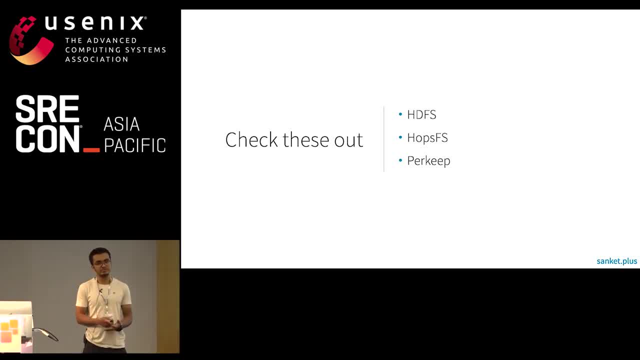 say three-node, and you've got active-standby configuration for metadata node. So that is how you do the HA part. What HopService did differently is you get out of the journal node. Instead you put a MySQL cluster. So in MySQL cluster your data is replicated. 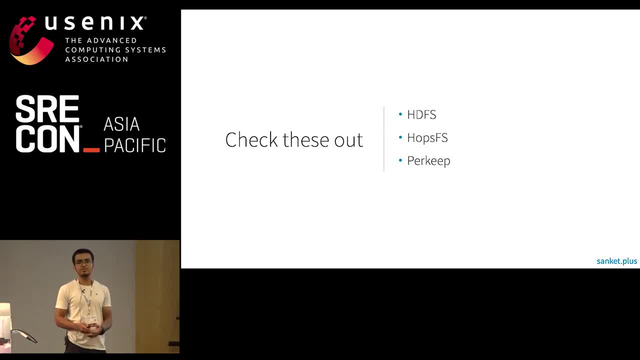 so that thing is taken care of, and now you can have multiple metadata nodes that are named nodes in HDFS nomenclature and they can solve your metadata requests. What Perkube does differently here is you don't have a concept of metadata or the metadata node. Where do you put your metadata? Well, you put it along with your data blocks. So, on the data nodes- say in this case minions- you'll be putting data as well as metadata. How do you differentiate them? Well, if you read a block, 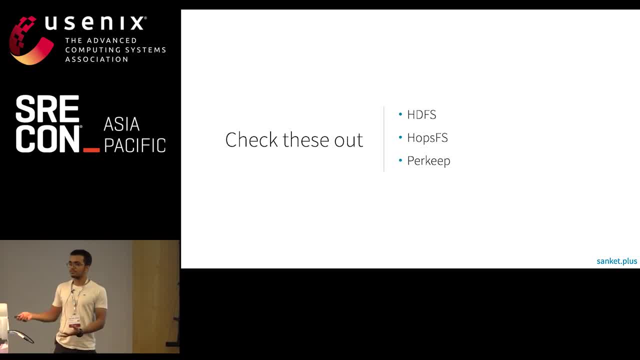 and if it conforms to some specific JSON schema, it is your metadata. So that is how you read all the blocks. If the blocks conform to a specific JSON schema, it's your metadata block. You read all these metadata blocks and you can create a file system index. 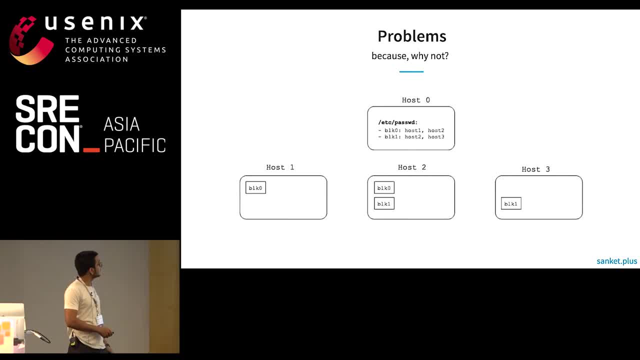 and that you put on metadata node. So you read all these blocks and if they are found to be metadata blocks, then you know it is metadata and you'll be putting it on metadata host. So you create an index. So if something happens to metadata node, 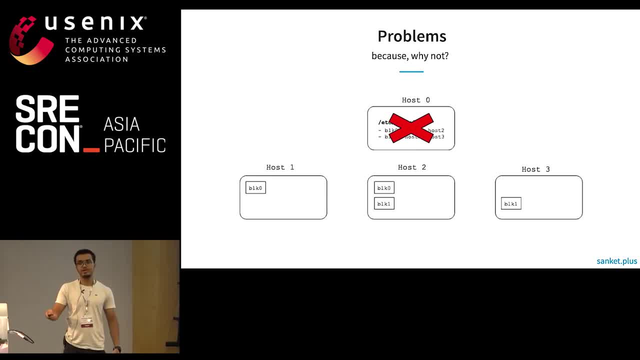 if it gets wiped out, you can always go read all these blocks, figure out what are the metadata blocks were and recreate the index. So that is how Perkube does it If data host goes down, in this case the Minion. 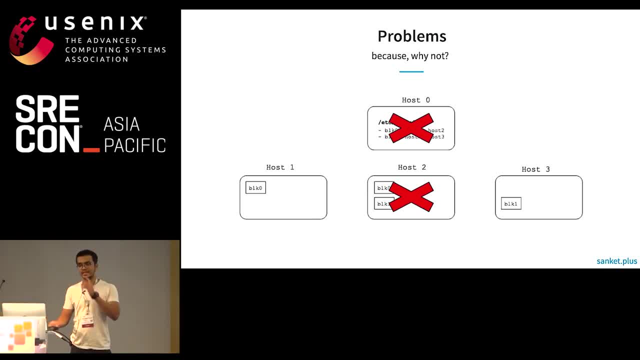 well, because you got multiple copies, they can come back up and join the cluster again and you got your application factor maintained. If some cases happen that this goes down or crashes and it is not recoverable, file systems also handles that by adding some complications. 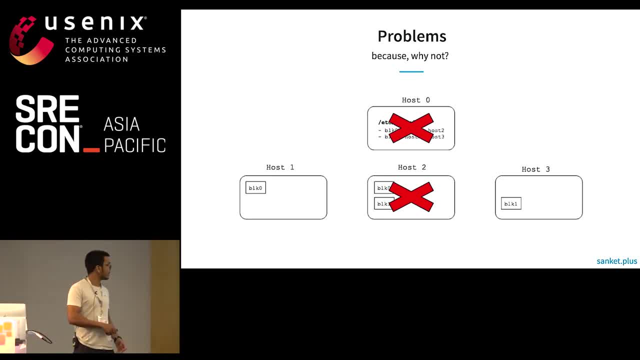 so we'll not go there. If you're interested, we can talk about it later. Now, these are some problems. There are some limitations. of course, This is not one solution for all your problems, So these are some of the latent problems. 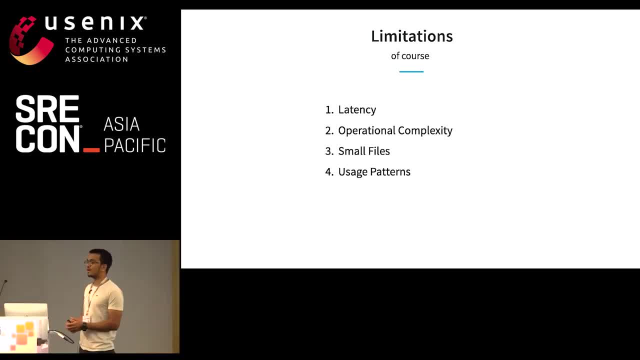 the first being latency. Why What we did? How did we make it distributed? Well, we took a bunch of hosts, put it on a network. So what we introduced here is network, and with network come uncertainty, latency, things like that. 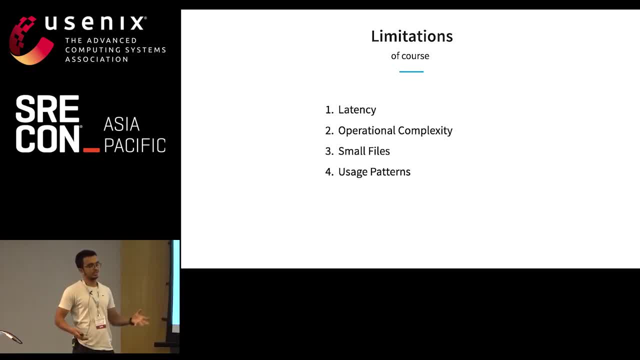 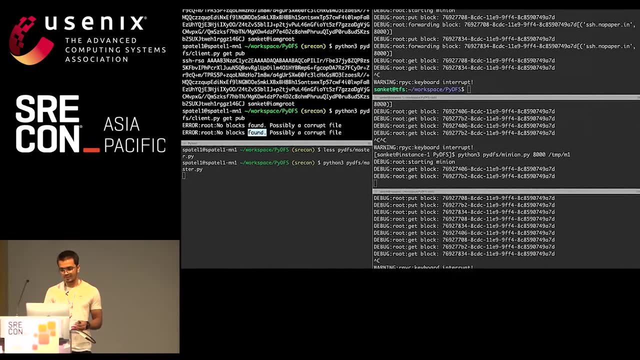 So now when you read a single file, you go to metadata host first. you jump networks so of course there will be latency. So we saw in this example as well, right? So if you read a file, see how long it's taking. 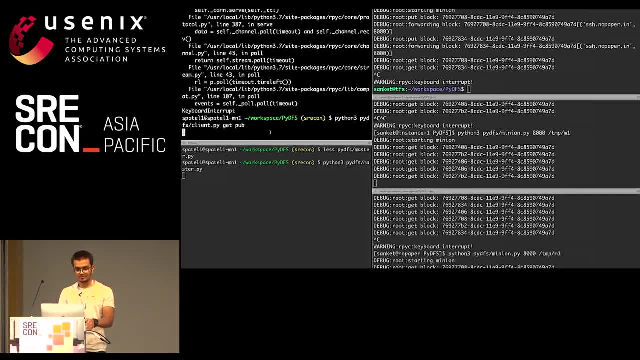 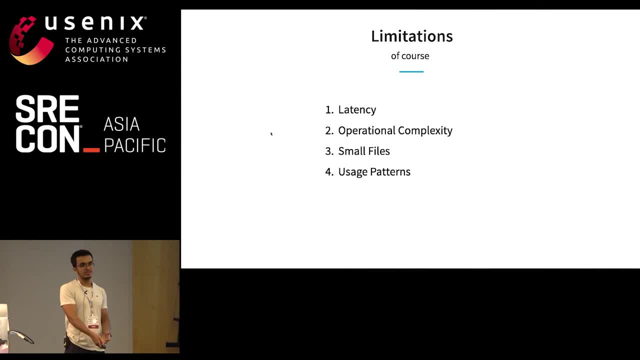 It's taking in seconds. right, Because this is distributed across cloud. but even if you put all these in same data center, it won't be as fast as your local disk. So latency will be there because they are distributed across networks. 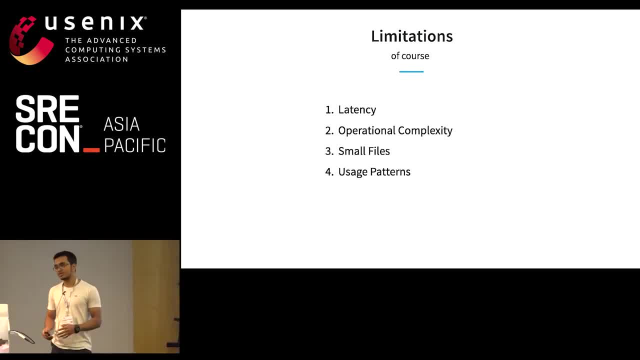 There will be operational complexity as well, Because earlier it was a single disk. maybe a driver will be there that is there to access. Now you put it on different hosts. Now your file system is distributed across hosts, So you have configuration management to do. 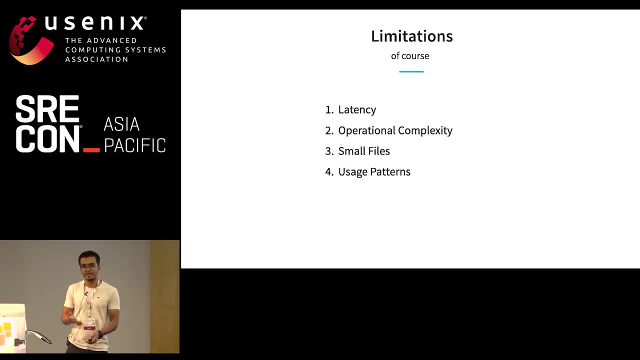 You need to make sure that they are all version compatible. You need to maintain their uptime, So it will get operational complex. You need some special people or team set up to maintain this. If you want to look at the components, you see this. 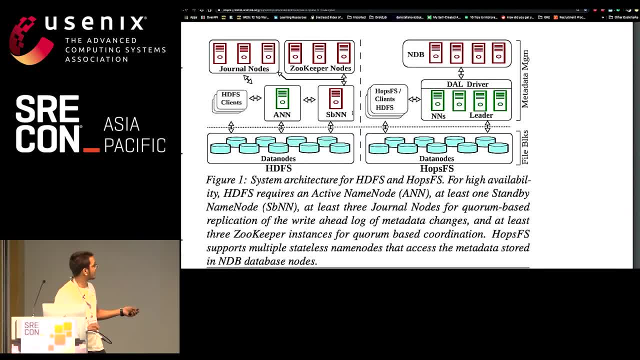 This diagram, on this side of the dashed line, is the HDFS. So you see there are data nodes, There is a name node, active name node, standby name node. To maintain the active-passive standby, you also need to operate a Zookeeper cluster. 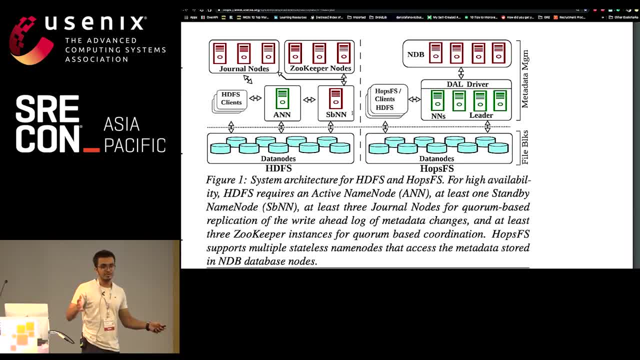 You also need journal nodes, So tons of components that you need to manage, So this gets operationally complex. In case of HopsFS, you can see there's, instead of journal nodes, there's a MySQL cluster and you have n number of metadata nodes. 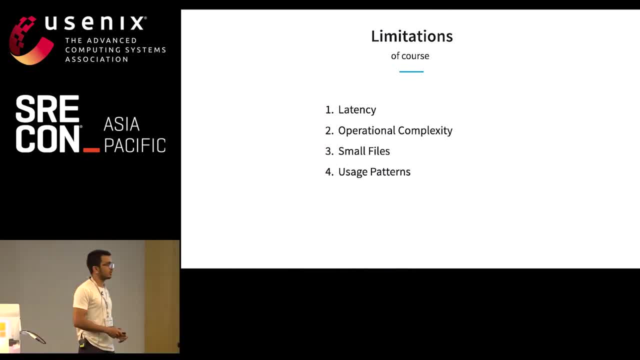 So it gets operationally complex. It also doesn't work well with small files. So in the demo we saw it was a really small file. But if you are to put it on a distributed file system it may not be optimal because to read a really small file. 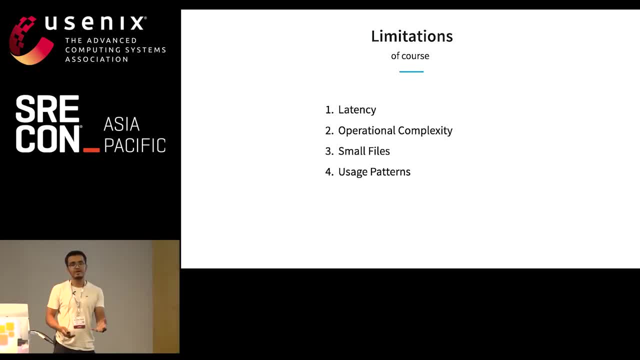 you need to go to two, three hosts. you go over a network and then finally get a small file. Also, you'll be using a lot more metadata space because you've got limited metadata space, because you've got only one host or n number of hosts. 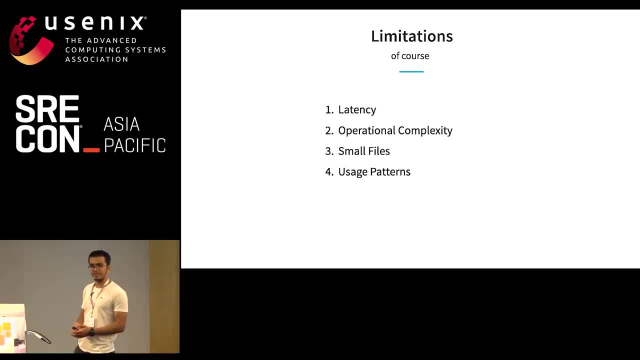 less than data hosts, So they'll be consuming memory, So you may not want to put a lot of small file. It doesn't work well with small files. And last, but it's not an exhaustive list, is this patterns? So we talked an example of LinkedIn's dataset. 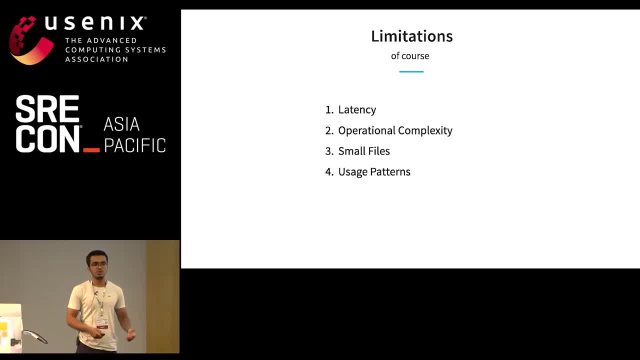 We'll be reading file. Ten people are reading file in parallel, So in those kind of cases this thing scales well. You can create instead of ten. you can create 20 copies and reads will scale as well. But if you wanted to write to this file, 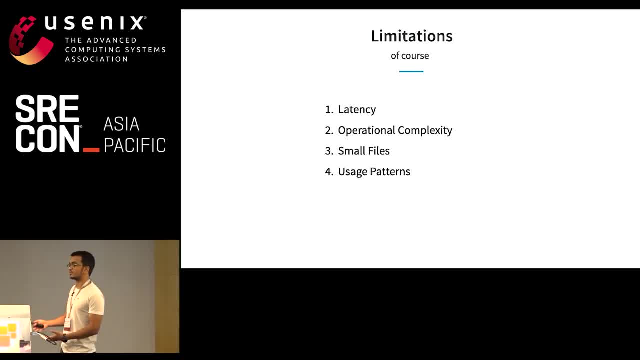 ten people are simultaneously writing it to this file. Then all these distributed systems concept. you want to maintain consistency and things will start to get more complex. So it does not really do well with the random writes cases. So that is why HDFS also takes a lot. 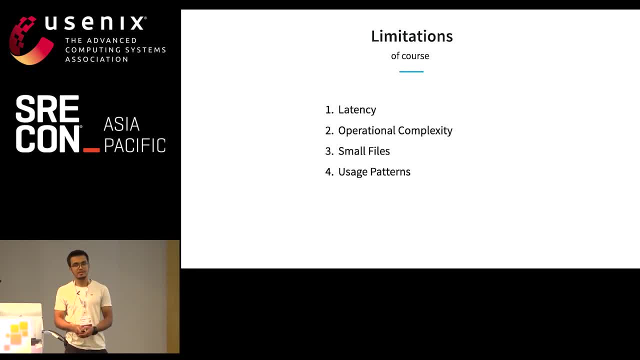 and restricts you to either append or read. You cannot write at any random place in the file. So these are some of the limitations and these were distributed file system. I hope you learned something here today, and that is all from my side. Thank you. 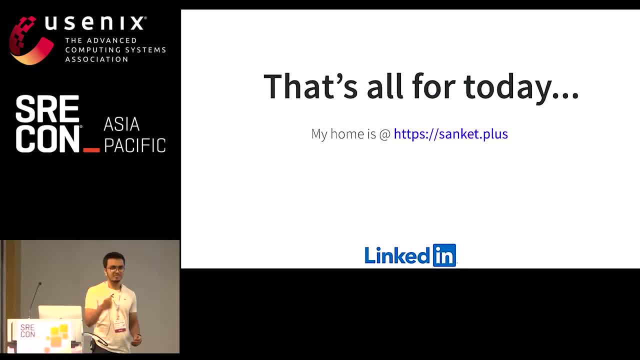 This is my home. If you want to look me up, tweet me any feedback, whatever Questions. Yes, If you got any, So my queries. let us say that I am writing and reading the file at the same time, So what exactly happens? 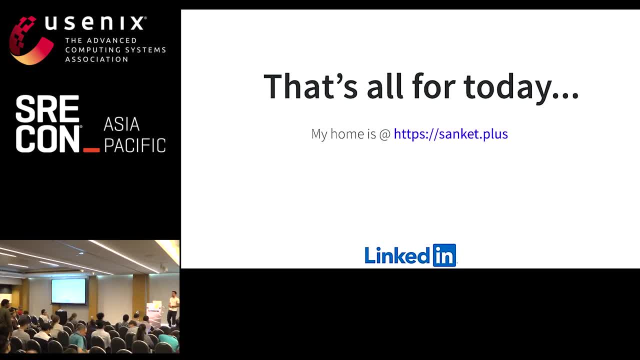 I am trying to do. Let us say that I am trying to write a large file And one of the client and another client is reading the same file. So how exactly my behavior will be Writing and reading at the same time. So metadata. 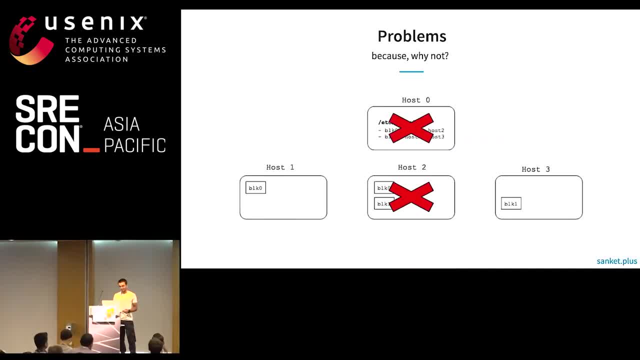 so that is what, If you go back to this diagram, so it can happen that file is being written. and it also can happen that you wrote it on host one first and host two was down, so it was not written. It can happen, right. 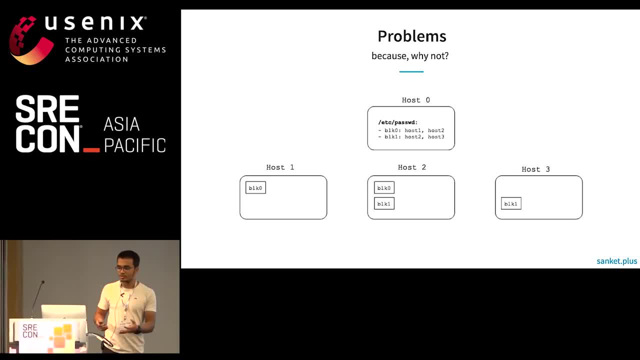 You are creating multiple replicas. So what? this was simple implementation. but in real case metadata node will be keep tracking of these blocks. So if block one is written on host one, host one will be sending some reports to metadata node. So it will tell that I have block zero on my local disk. 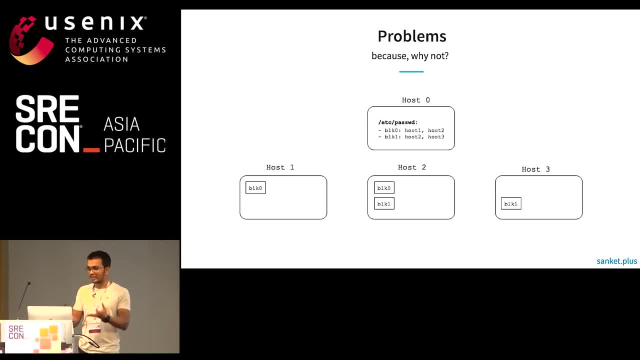 Host two will be telling I got these two blocks. So this is how metadata node will be, knowing that these are the blocks that are supposed to go, that these files being written, these two blocks are supposed to go, And in the reports it has got only one block. 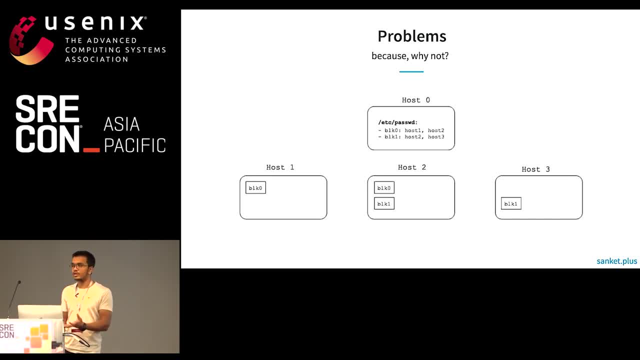 So it will know that this file has not been written yet, So metadata node can contain, can kind of maintain, the state that where exactly is the process? how are the blocks, how many blocks are there, how many are missing And in case, if it goes missing, 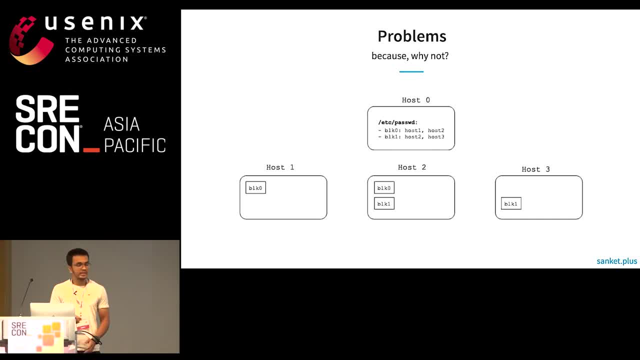 say, this host went down and it never came up. so in the reports metadata node will come to know that only one copy of this block is getting reported, So it's kind of under-applicated. You're following, Yes, yes. So finally, 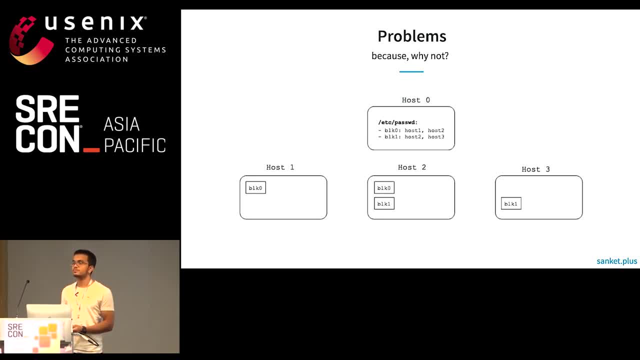 like the client. let us say that, in that case, let us say that three blocks has been written. Let us say that, okay, the file is not serving three blocks, So let us say that first block has been completed. So let us say there is another client. 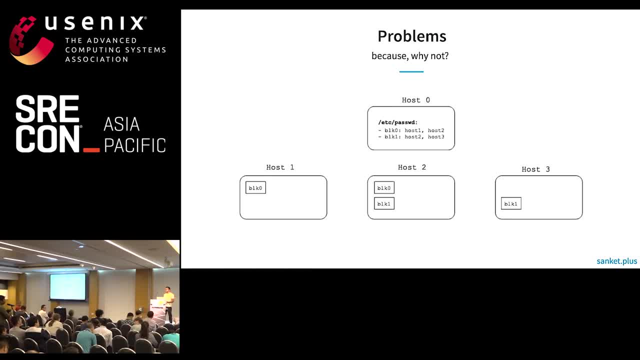 that has been asking for the same file at that time. So will it be showing the first block content or it will not be showing like error? So it will depend on what file system implementation you're talking about. In general I'm not. 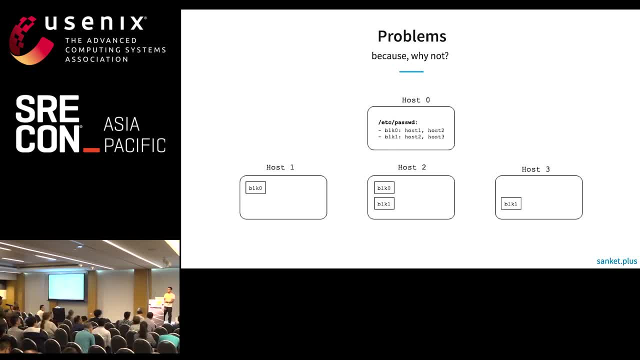 It's not in general. So if you are to implement a file system, you can enforce that once file has been written, then only you can read. So you can implement it that way that once it has been written all the blocks are reported. 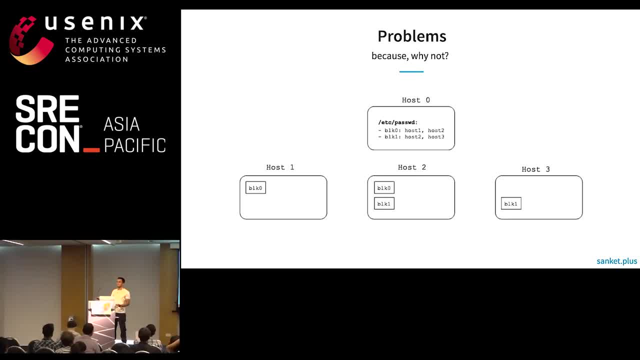 they are confirmed to be written, then only read operation can be allowed. That can be done. It depends on the file system. That's what I'm saying. Okay, It might be a long question. Can you just give a brief idea, like how the access control or security? 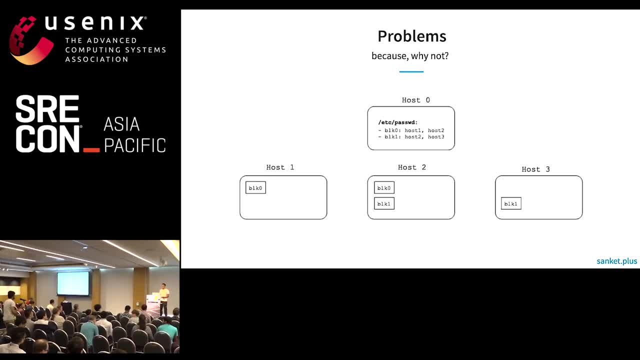 is maintained in distributed file system. Yes, So that is also implemented at the metadata host. So, because you are In this diagram, we are simplifying things a bit and we just have file to block mapping, But along with that you can also have user sort of information. 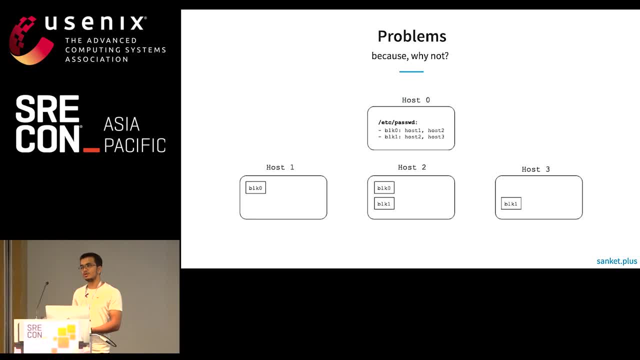 that you have in normal file system, that who is the user of the group, So those sort of concepts can be introduced here. So this is the place where you put your access, control and those kind of things, Ownership And one more thing Like in your diagram. 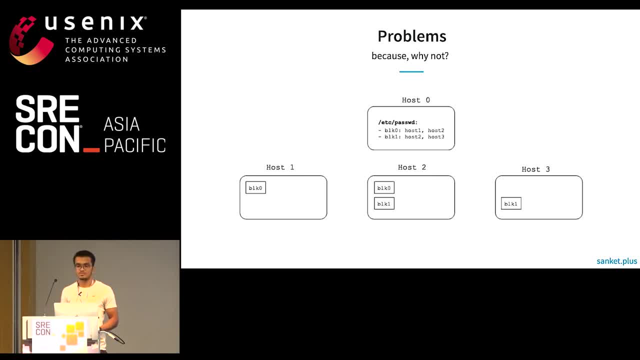 like you showed that direct Clients have direct access to all the hosts, right, Yeah, Yeah. So is it like pretty common like way to do it or like mostly like there are like some kind of proxy server? No, As far as I know. 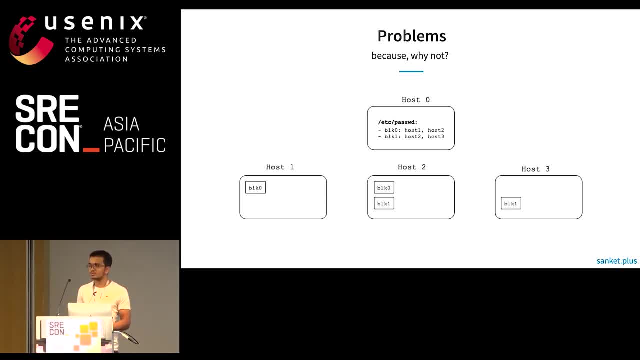 they go directly the clients. They go directly to the data hosts. So authentication methods are there, that Kerberos or those kind of things can be used. But if you start up a cluster and do a real basic setup, you'll be going directly.